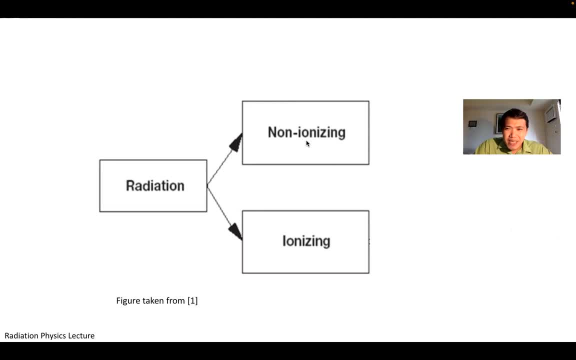 from the word itself. It cannot produce ions, It cannot destroy DNA, It cannot destroy chemical bonding. But if you talk about ionizing radiation, if a molecule is being hit by an ionizing radiation, it can damage the molecule, It can knock off electrons. So usually the molecule or the 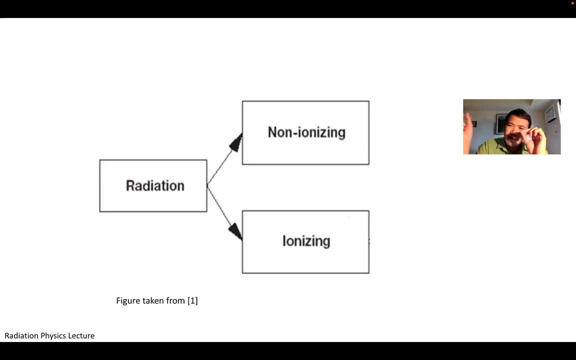 element is neutral, But if you remove an electron, it becomes positive and negative. So you produce two charges, You produce ions. You produce positive and negative ions. That's why it's called ionization, ionizing radiation. Okay, so what are the examples of ionizing? So we have x-rays. 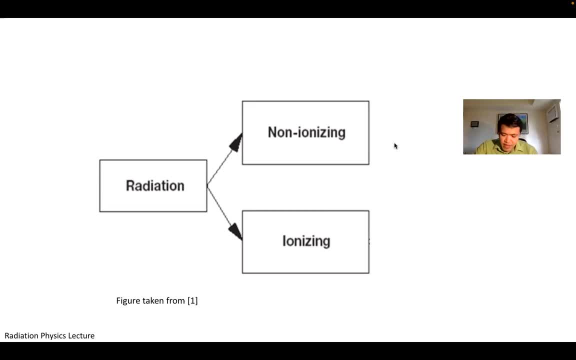 gamma rays, some part of UV And proton type of radiation can be ionizing. Particle type of radiation- Neutron- that are fast moving, very high speed. neutron Electron can also be ionizing fast moving. Okay, what about non-ionizing, Non-ionizing radiation? these are radio frequency. 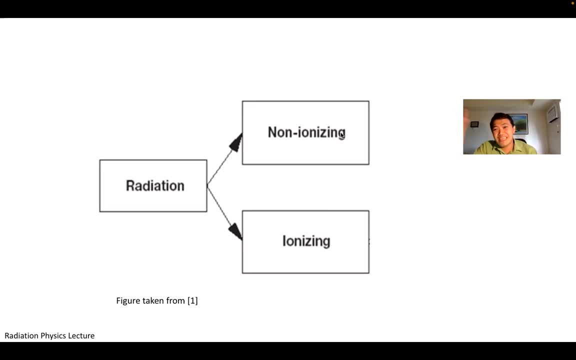 from your cell phones. It cannot cause DNA damage. It doesn't ionize Your DNA. Ultrasound, although it's not electromagnetic, it's mechanical type of radiation. Ultrasound is non-ionizing. Okay, what else? Visible light is non-ionizing. So if we're 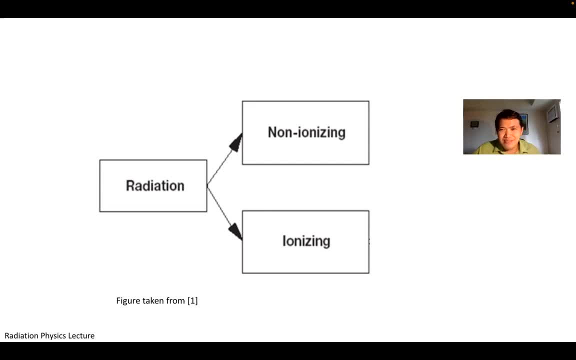 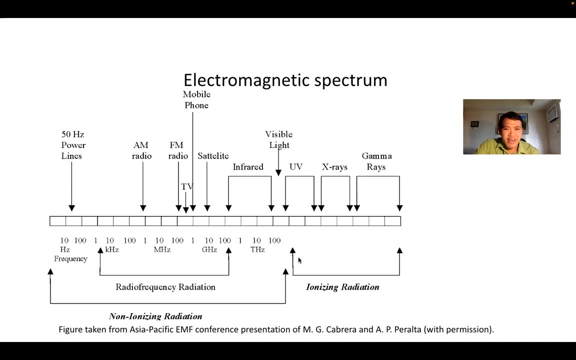 being hit by visible light like here, don't worry about cancer or whatever. It doesn't produce ionization, It's non-ionizing. Okay, so let's go now. There's a nice photo here about the separation of ionizing and non-ionizing. 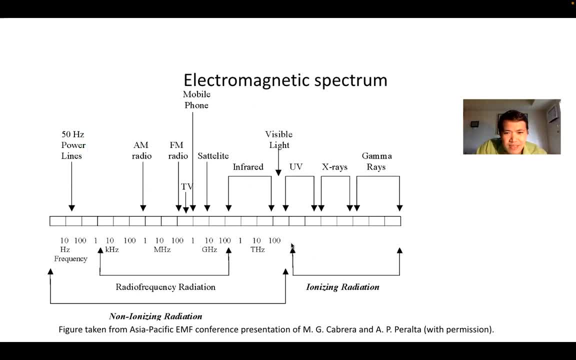 So, as you can see here, so ionizing here, from UV to x-rays and gamma rays, Non-ionizing visible light, infrared, the electromagnetic waves used in FM and AM, even in your cell phone microwave, these are non-ionizing radiation, Even your power lines. In the Philippines we use 60 Hertz power. 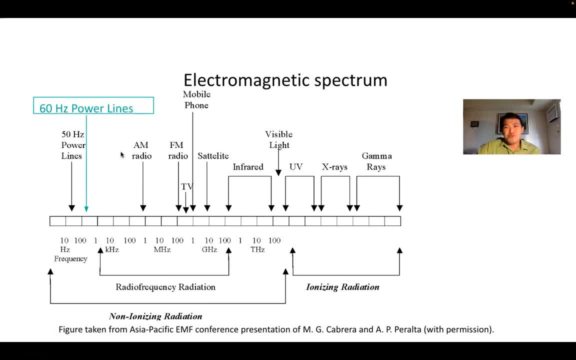 line. It produces radiation, but it's non-ionizing. So we are all exposed to radiation, But non-ionizing, it's mostly non-ionizing. Okay so your wires, if it's connected to your current. it produces radiation actually, but on the lower spectrum here on the left side. Okay So AM FM satellite. 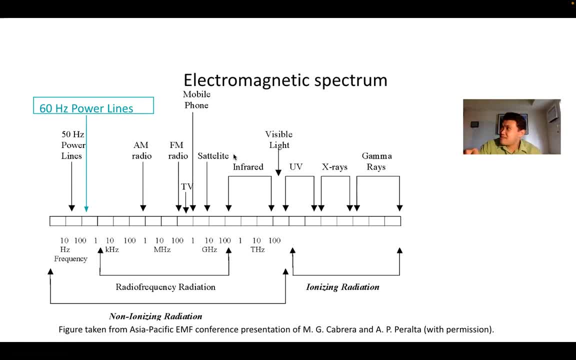 infrared. non-ionizing Microwave, the one that you use when heating food, is also non-ionizing radiation. It cannot ionize, Although most of the non-ionizing radiation the effects are, especially in infrared and microwaves. the effects are heating. it can cause heating okay, even visible and for uv. 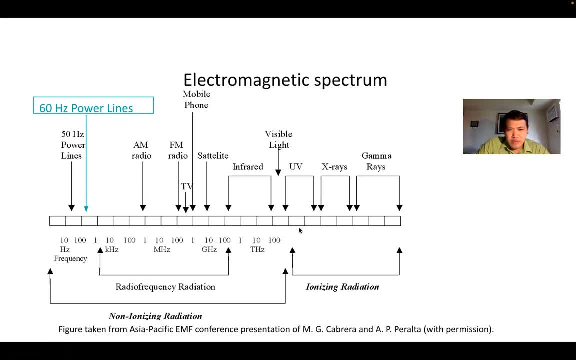 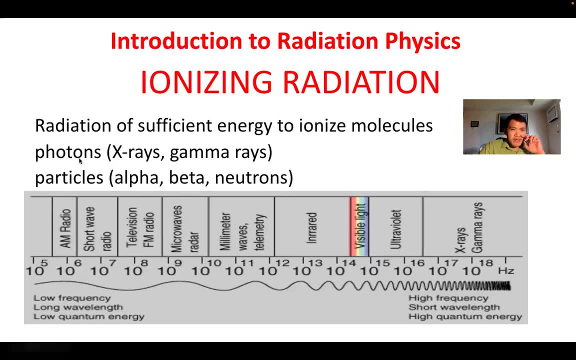 that's the part border where you you will have ionizing radiation, okay, so if you're going to look at this figure here, ionizing radiations are radiations of sufficient energy to ionize molecules. examples are for photons, electromagnetic as well, x-rays, gamma rays, for particle type of. 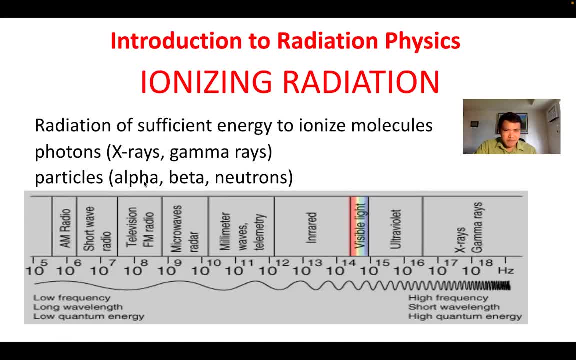 radiation. these are fast moving particles. examples are alpha, beta, neutrons and even protons. if it's moving very fast it can be an ionizing radiation. so let's go back to your electromagnetic waves. so these are lower frequency on the left and you have a longer wavelength, but as you go further to the right the frequency becomes. 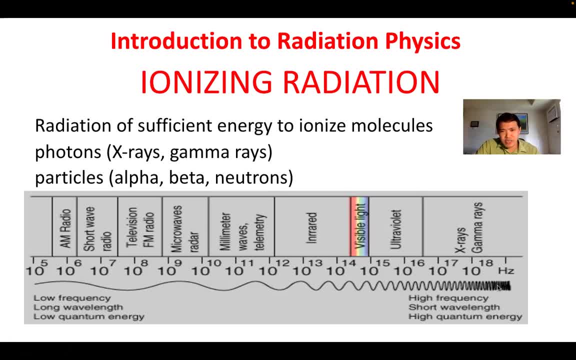 higher, but the wavelength- wavelength of light- becomes shorter. can you imagine? this is the only part, what? of the electromagnetic waves that we can see. the rest we cannot see, we cannot smell, we cannot detect, unless you have a detector. okay, so now let's go to. so let's go to. let's d, let's uh. 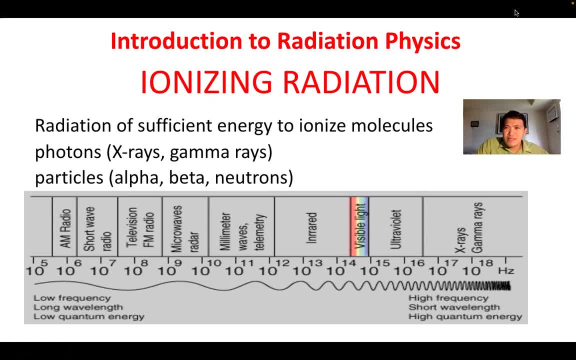 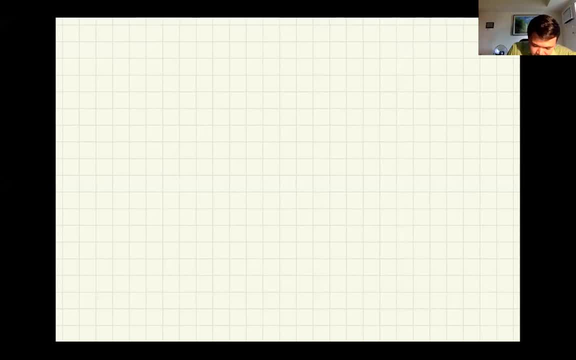 define ionization. okay, so what is happening in ionization? so let's say you have, uh, an atom with a nucleus. let's say you have neutron here, your proton there, so there can be a lot of them. and then let's say our classical model right of of an atom, this is your orbit of the electrons. so let's say we have 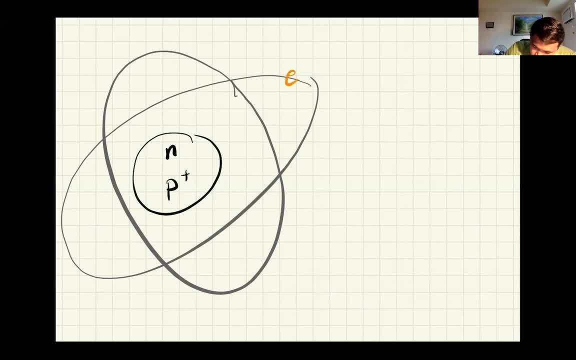 here, so negatively charged and your electrons orbiting around another negative. but what if you have a, an ionizing radiation hitting the electron? so let's say this can be x-ray, some part of uv, gamma ray or particle types of radiation such as even fast-moving electrons. 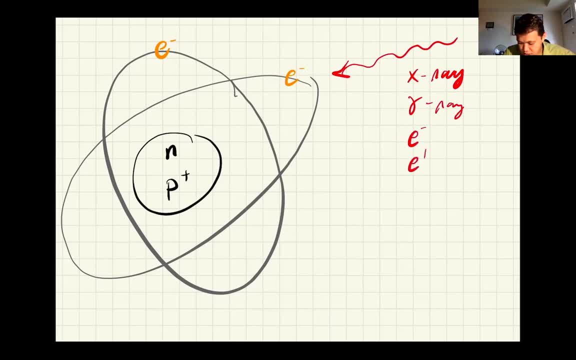 can be an ionizing radiation. there is also a positive electron we call positron, or a fast-moving neutron, no charge, or a fast-moving proton and other cosmic radiation particles. okay, so these are actually particle, particle type of radiation, and these are electromagnetic waves or or a photon. photon is like a pure packet of energy, no mass, so 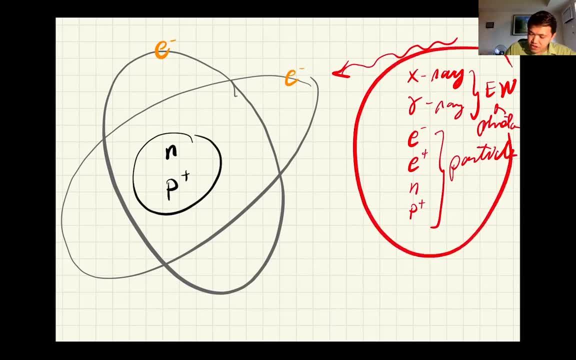 they are highly energetic, this ionizing radiation, or highly energetic type of radiation. they can knock off electrons, they can remove electrons out of its orbit. so later on, after the process, the electrons will jump or not jump, but will get moved on the orbit. and so this whole. 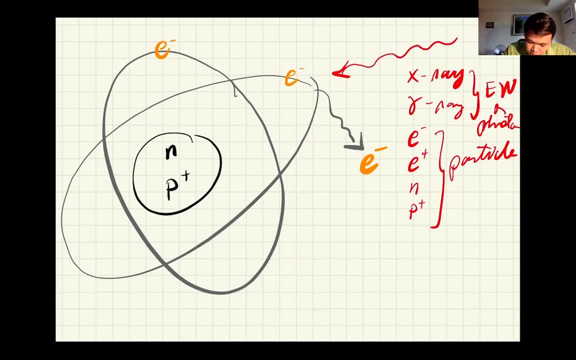 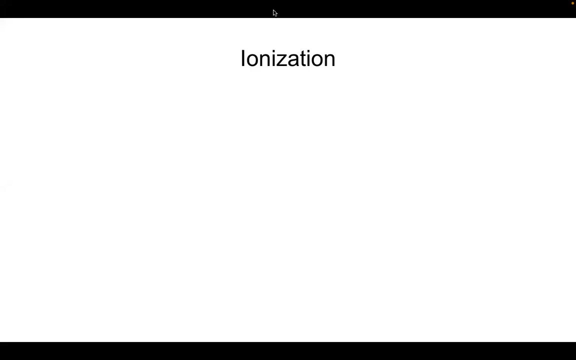 atom will be left with an electron, so it will. it will become a positively charged. so you actually produce ions, a negative and a positive, positive ion. so ionization is the process of removing an electron from its orbit, from the outer shell. okay, so, as i've said, our radiation is actually all around us, but now let's focus on ionizing. 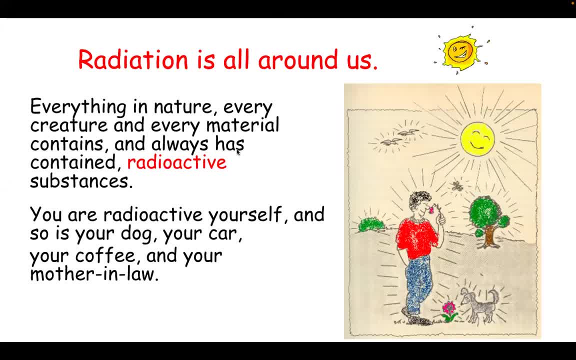 radiation. let me read this. i'm- uh, this is a slide during my masters. radiation is all around us. everything in nature, every creature, every material contains, and always has contained, radioactive substances. you are radioactive yourself, and so is your dog, your car, your coffee, your mother, your mother-in-law, everyone, everything. 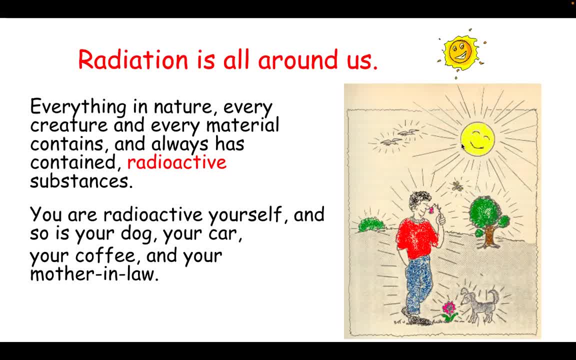 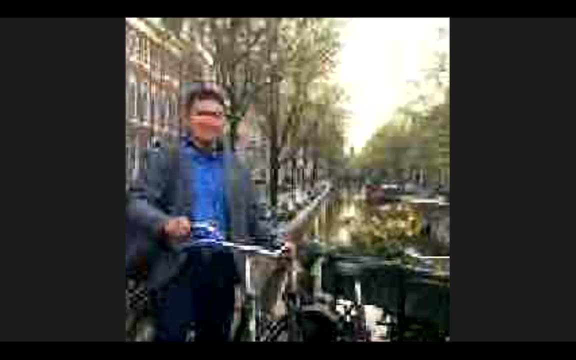 has some form of radioactive material. okay, so you cannot actually escape ionizing radiation because they are all around us, radioactive substances that emits ionising radiation is all around us. okay, banana that you ate for breakfast earlier banana has a potassium, that is a radioactive. let me so, if you, if you have a sensor, let's say a geiger counter, let's say: this is your. 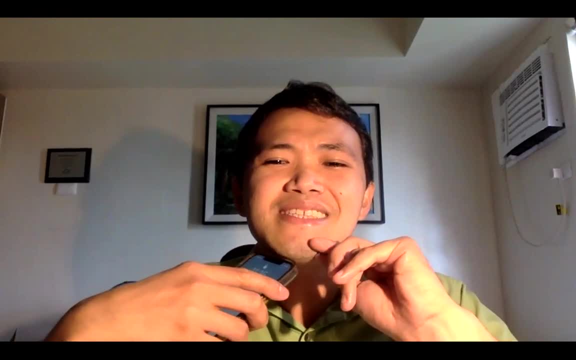 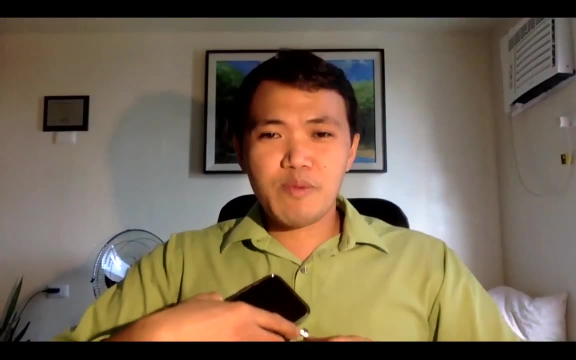 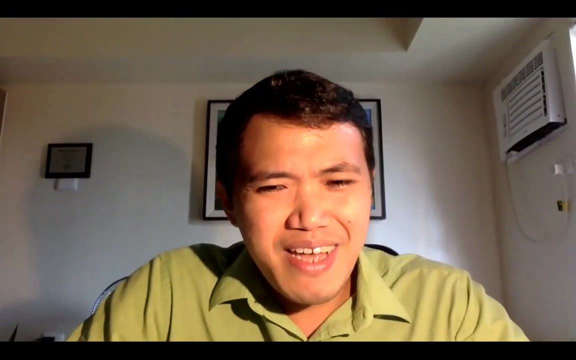 geiger counter and you eat banana, you can actually detect the emission of this radioactive material. if you eat banana, you can detect it using a Geiger counter. So it's amazing. right, You're actually surrounded, But you know the levels of. 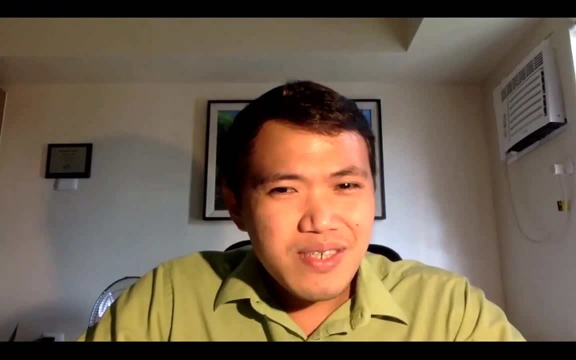 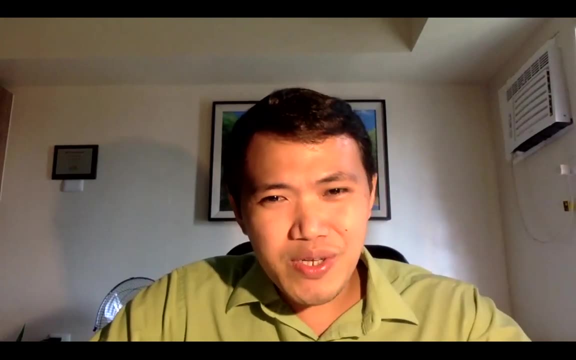 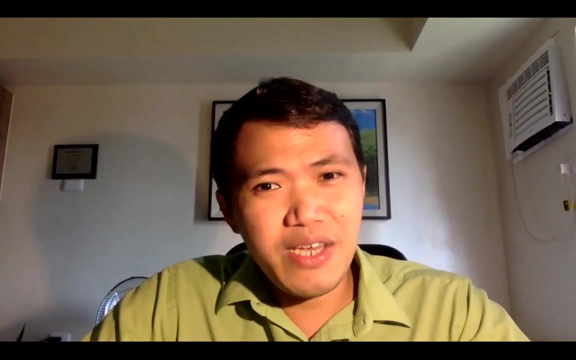 this ionizing radiation is low, so we can consider them as background radiation. Everyone is exposed to this background, but if you're exposed more to, like artificial sources, man-made, or the radiations, the radioactive material that they use in the hospital, these are high intensity or higher activity. I will 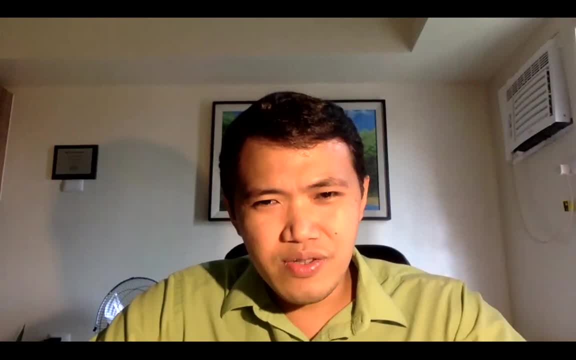 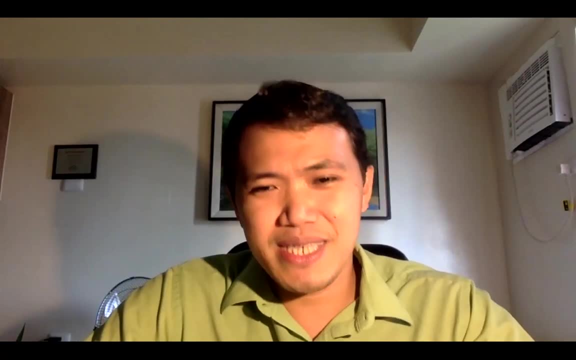 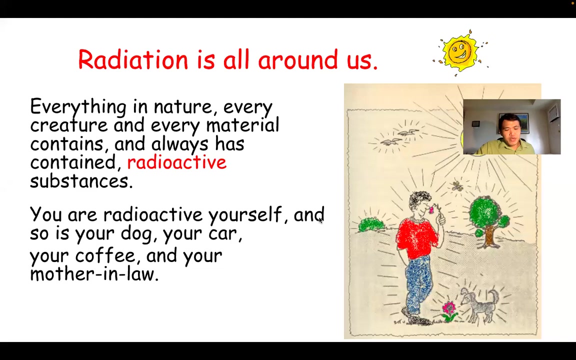 discuss that later. So there are more emissions on those sources of radiation. So we are not gonna expose ourselves to that unless we need it for medical purposes or medical application. Okay, so let me go back to my slide. So it's everywhere. 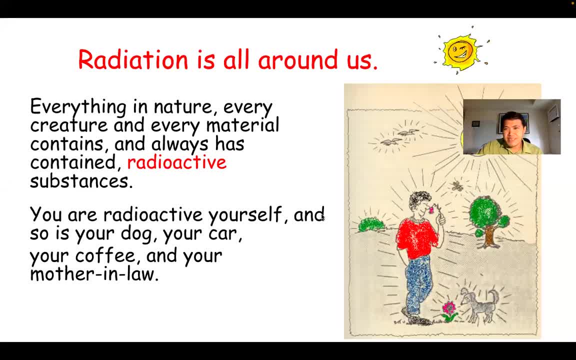 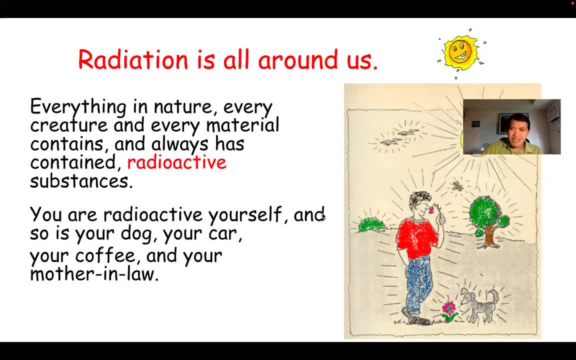 plants, from the food, from the cow. they will eat the grasses and they will have carbon-14. So we're gonna eat, drink their milk and then we will have carbon-14 in our body as well. So it's on the water that we drink. There are also other other. 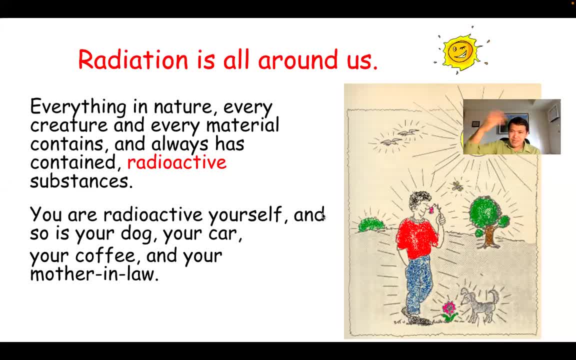 sources from the ground. Uranium is usually the ground, okay, and the minerals, and even radon gas from concrete. So my concrete here is some radon gas, but so once in a while we open the windows, but it's very minimal, guys. Okay. but just to tell you, ionizing radiation is all around us, Okay. 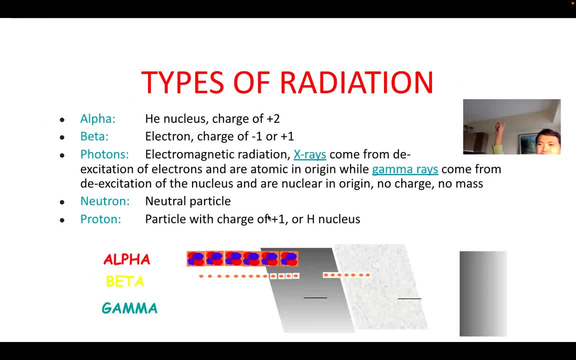 so, if you're going to look, I have a smoke detector and if you can see it, I have a smoke detector and it uses an alpha emitter radioactive material. So let's go to the different types of radiation. So there is an alpha, just actually a helium nucleus. 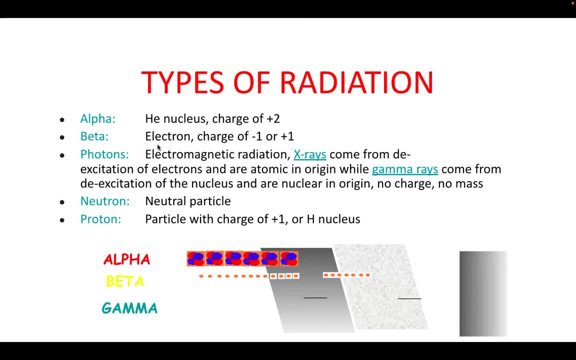 and with a charge of positive two. There is beta, which is actually an electron, with a charge of negative one, or an antimatter. beta positive one- We call it positron, positive electron and photons. photons are electromagnetic radiation, such as x-rays and gamma rays, so x-rays came from. 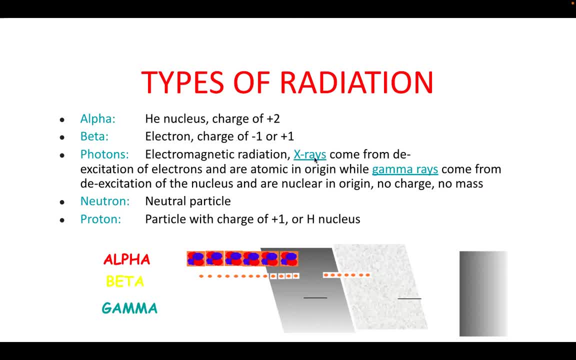 the excitation of electrons. we usually produce it with a machine right x-ray machine and gamma rays. this comes from the nucleus from radioactive material, from the nucleus of a radioactive material. it has no charge and no mass. both x-rays and gamma rays have no charge and no mass, as 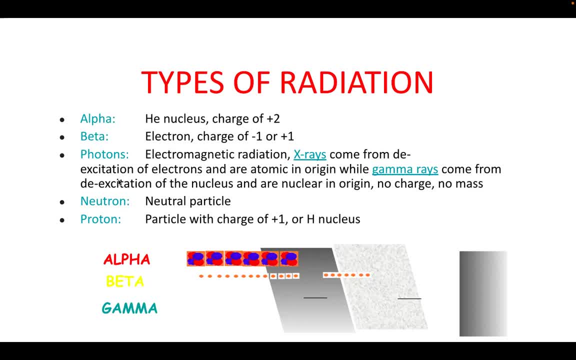 compared to particle type of radiation. alpha, beta, neutron and proton has mass, okay, different charges, but all of them has mass, except x-rays and gamma rays. neutron is a neutral particle, proton a particle the charge of positive one, or a hydrogen nucleus. now we can shield aqua particle with just. 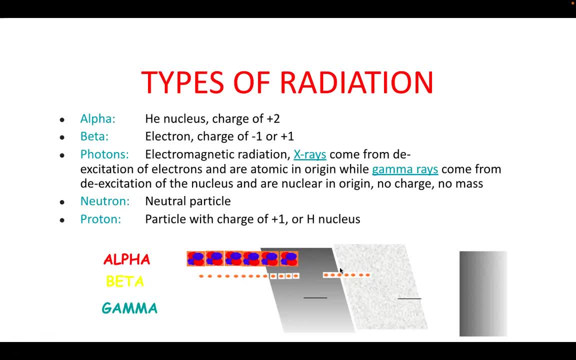 a piece of paper. beta can pass through a paper and can be shielded by aluminum. definitely concrete gamma cannot be shielded by paper, cannot be shielded by aluminum. not much can still penetrate, and even concrete. so gamma, radiation and x-rays can still penetrate concrete. but 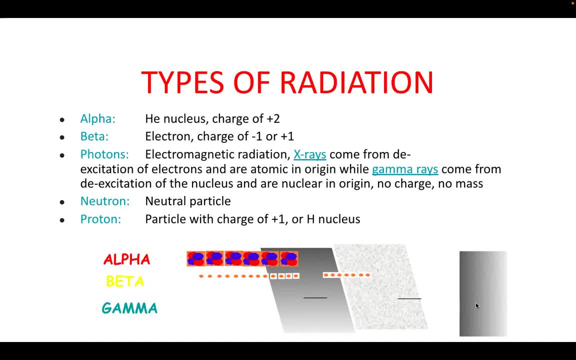 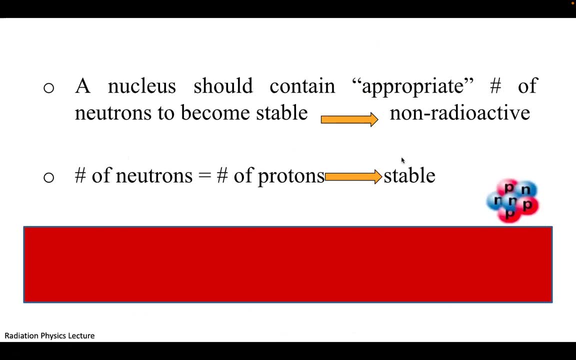 if you have a steel, and especially lead. lead can shield gamma and x-ray radiation. okay, so let's go back to radioactivity. so radioactive happens if the nucleus of your radioactive material or the element. the nucleus has proton and neutron right to be stable. they should be equal. 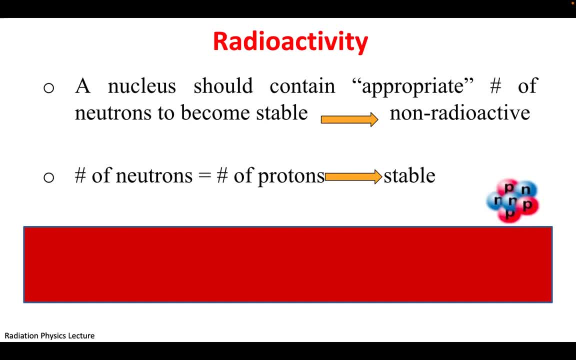 but if the nucleus and the proton inside the neutron and the proton inside the nucleus is not equal, they become unstable. okay, a nucleus should contain appropriate number of neutrons to become stable. non-radioactive. that means the the nucleus has e as neutron equal to the number of. 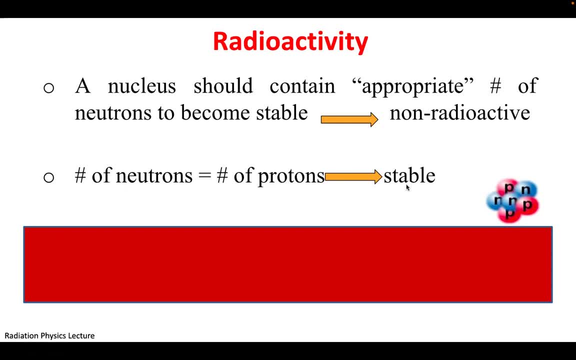 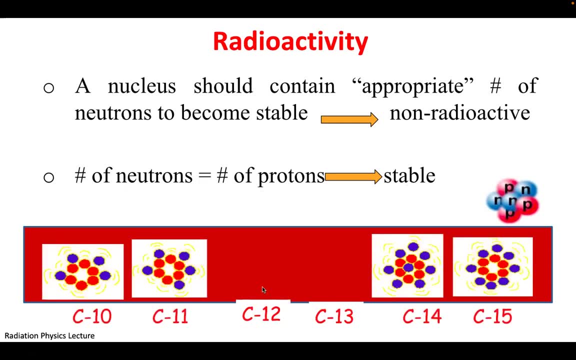 proton. the number of neutron equals the number of protons stable. if they are not equal, then they become unstable. so for example, for carbon: okay, the mass number is 12, so the number of neutron and proton is six. six neutrons, six proton, non-radioactive stable. 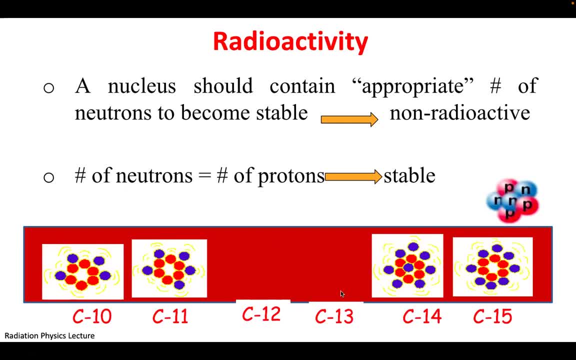 that's not good, because it's still stable, even if it has more- uh, more- neutron. now the proton is six, the neutron is seven, but as you can see here, this one lacks neutron, so there's an excess of proton in a way. so it's now unstable if the number of neutron is not equal. 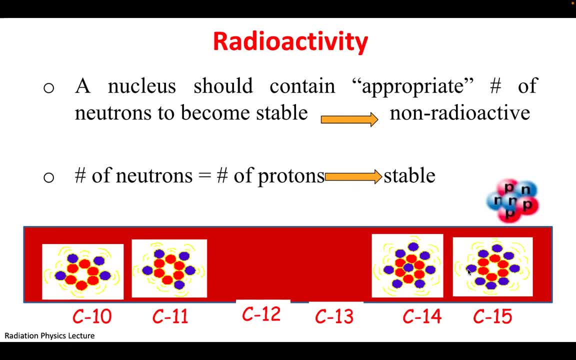 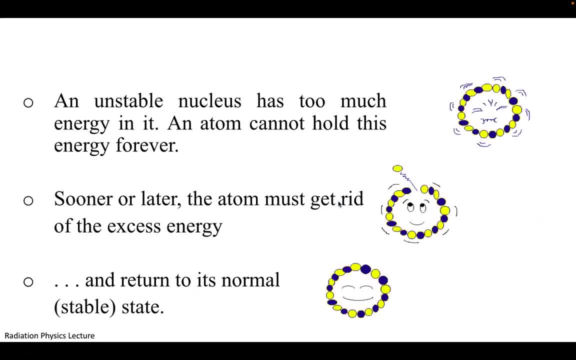 to the number of protons, they become unstable. okay, carbon-14 is unstable. carbon-15 is unstable, unstable. more neutral, more neutral, less. less neutral, less neutral. okay, an unstable nucleus has too much energy in it. an atom cannot hold this energy forever and it has to be ejected. 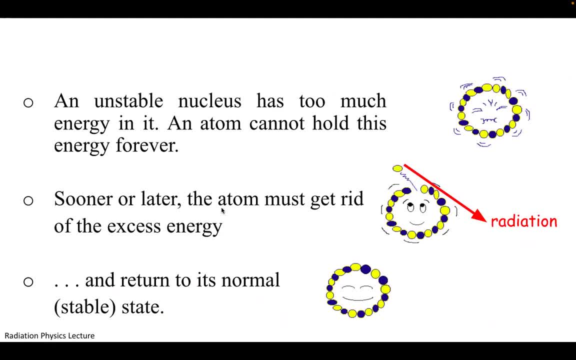 after some time, sooner or later, the atom must get rid, get rid of this excess energy, and that is through an activity, through an emission of radiation, radioactivity- it will emit the excess energy. if it's too much neutron, it will eject or emit the neutral and convert it. 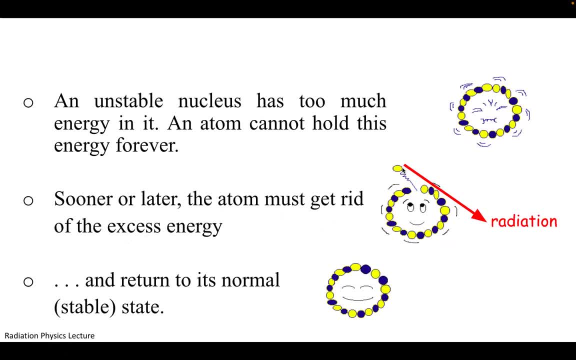 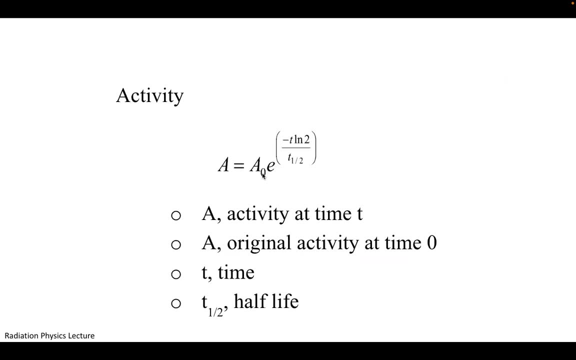 into another type of particle or a pure energy- yeah, radiation basically- and then if it emits these excess energy, then it will return to its normal, stable state, something like that. so this is the activity. as you can see here, the activity, the emission of radiation, is exponential. so activity now at time t equals the original activity times e raised to the negative t ln of 2. 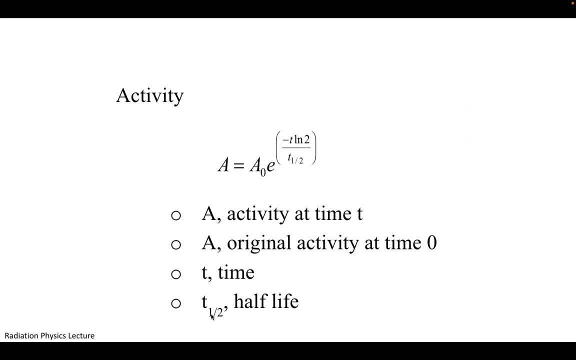 divided by the half life. half life is the time for that radioactive material, for its activity to be half of the original. so the time okay. so it's negative. exponential negative: it means it goes lower and lower. as time passes, the activity of radioactive material becomes lower and lower. 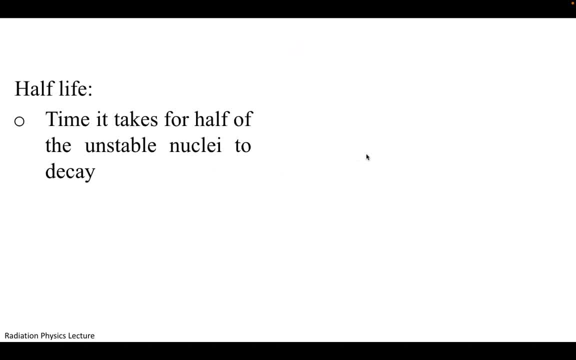 and lower. okay, so what is half life? half life is the time it takes for half of the unstable nuclear nuclei of the radioactive material to decay. so it means with each half life 50 percent of whatever there is will decay. so let's say time zero timer starts now. 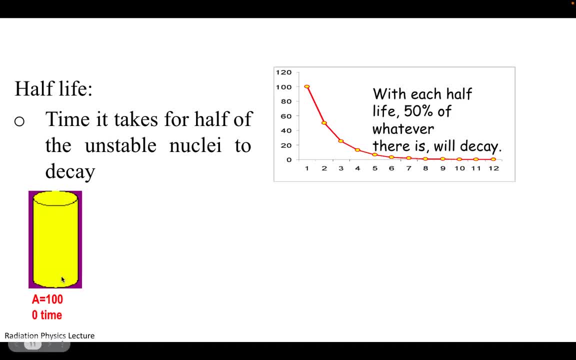 the activity is 100 after one half life. let's say that the half life is 100 years. after one half life, let's say after 100 years, the activity, the emission of radiation becomes half. so let's say originally after 100 years it will take half of that activity after another 100 years. 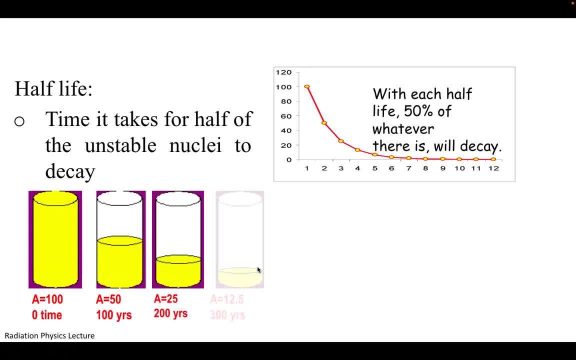 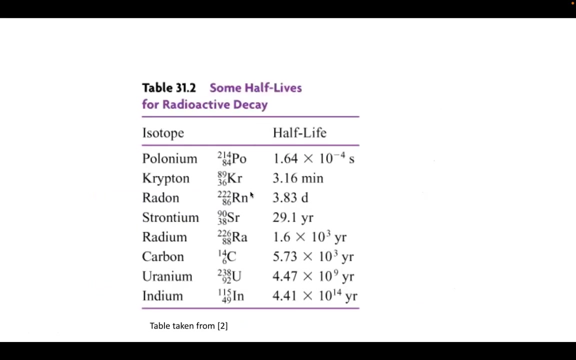 half of half, 50 percent becomes 25 percent after another 300 years. 25 percent becomes 12.5 percent with 12.5 activity and so on. so it is exponential. it goes down, down, down, down, exponentially. okay, so here are some of the half lives of some the common radioactive materials. 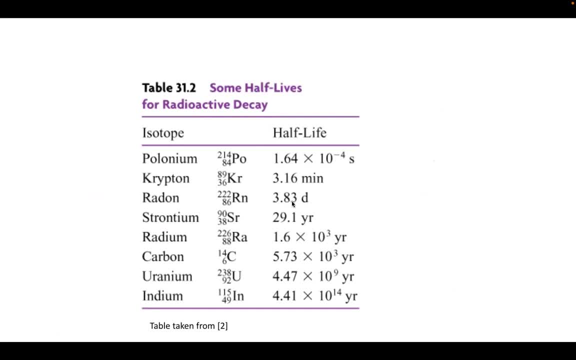 so polonium, krypton, radon- i told you earlier radon gas, radioactive material, but half life is 3.8 days- strontium, radium, carbon 14.. uranium is used to power nuclear power plants. some of these can be used as a weapon which? 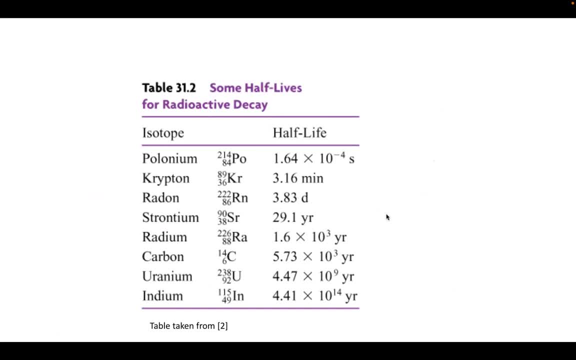 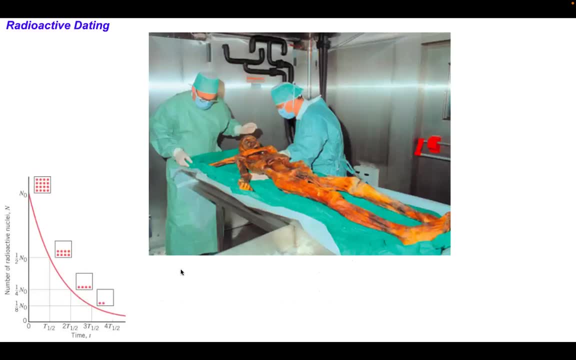 is not a good application of physics, you know weaponize, but some of these can be used to treat cancer patients to in research, let's say to carbon dating is one very good application because we can use this to determine the Loki effect. so we also tried to find monopetzenic filter. but the use of radioactive materials czy 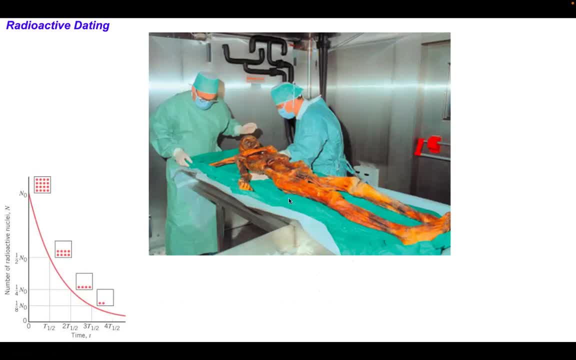 sokwehsoeto, member of Minnesota. is she ended up with sabes-mengou connectif mother sick virus was what? so i was wondering if you would describe in other languages with an example. i don't want to come for this. this is an example, but let us uh look at it in another, okay, so? 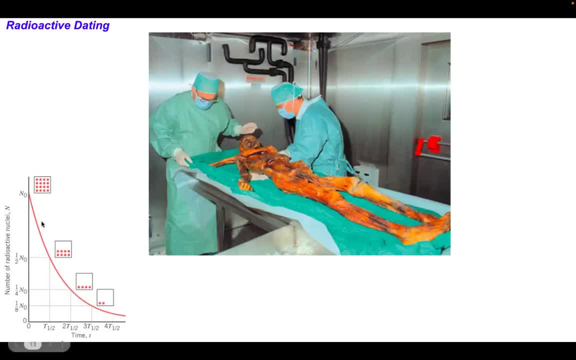 is there any? you weren't looking for that in Greater Tasmania, in Northuchshire. I can't. i just can't wait to talk about that because it's it's 5,000 years because of the activity of the carbon-14 emitted by the body and we. 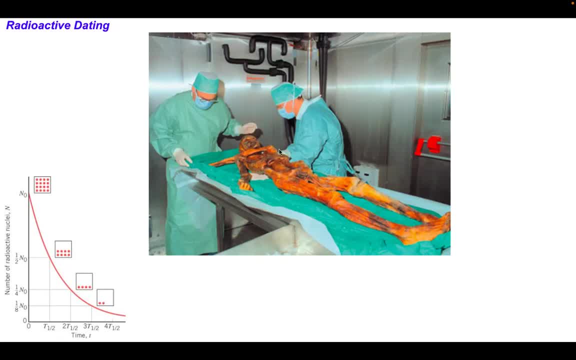 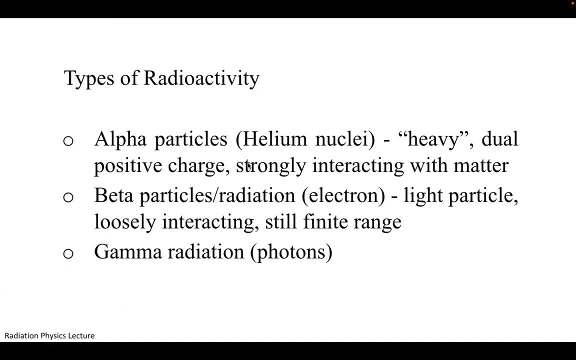 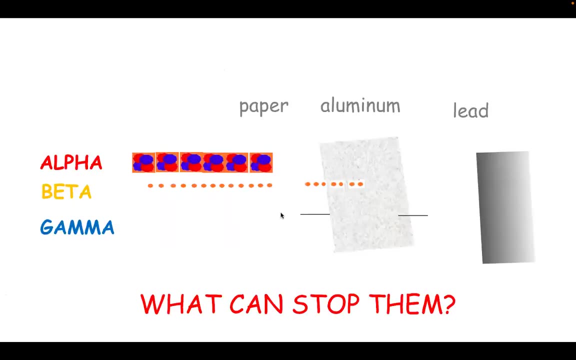 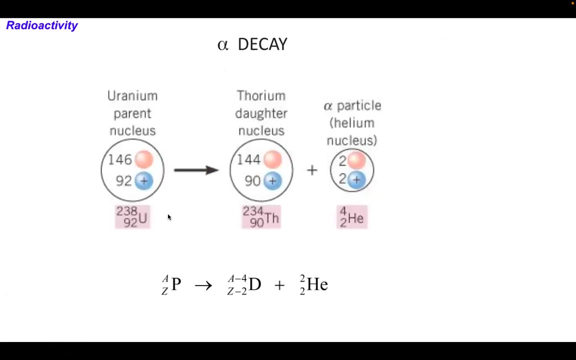 also have carbon-14 in our body. we can determine some Geiger counter measuring instrument. okay, so there are different types of radioactivity or the emission of radiation. there's alpha particle emission, beta and gamma. okay, so there is what we call alpha decay. so let's say you have a radioactive material, uranium. 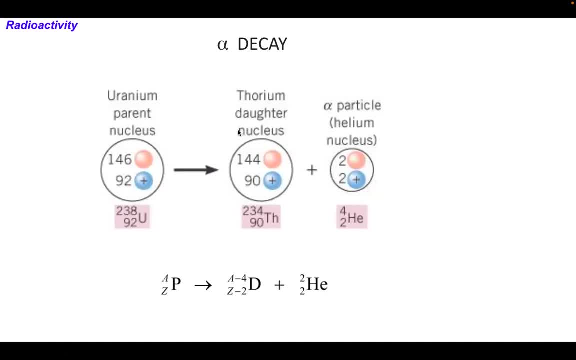 that's the parent. after some time it will decay. it will be stabilized a little bit, yeah. well, because it's unstable, it will go to its more stable state. okay, it will emit something, and that is, in this case, alpha. it will emit alpha and uranium becomes thorium. so this is the parent, this is the daughter. 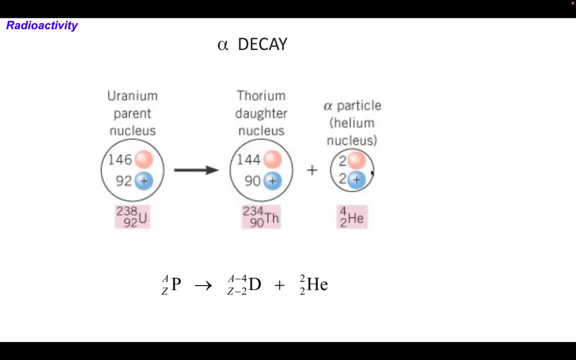 and this is the radiation that it will emit. so the mass number changes, the atomic number. this is the parent atomic number a, a mass number, a atomic number Z. after it undergoes alpha decay, the parent becomes a daughter. the daughter has a mass number of a minus 4. 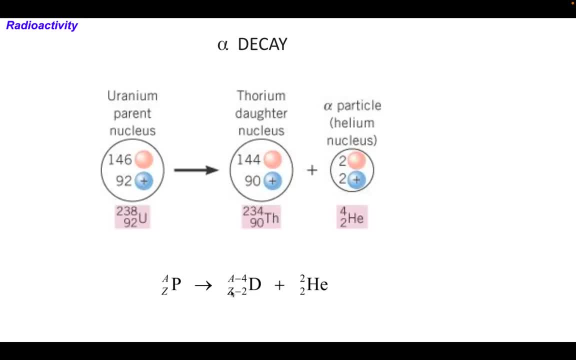 from the original 8 and the atomic number is Z minus 2, so 92 becomes 91, 46 becomes 1, 4, 4, plus the alpha that it will be emitted, that it will emit the alpha particle, which is an ionizing radiation. okay, so one application, smoke detector, as I've 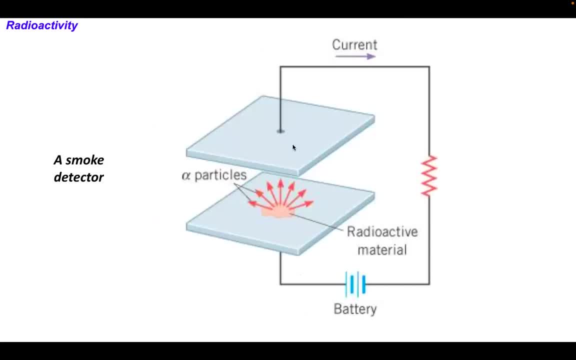 told you, I have a smoke detector. even I think in your house you have a smoke detector as well. so it's radioactive but it saves lives. it saves life. so what is happening? in smoke detector you have alpha particles and you know this is an electric circuit, closed electric circuit because it seems charges are flowing because this alpha 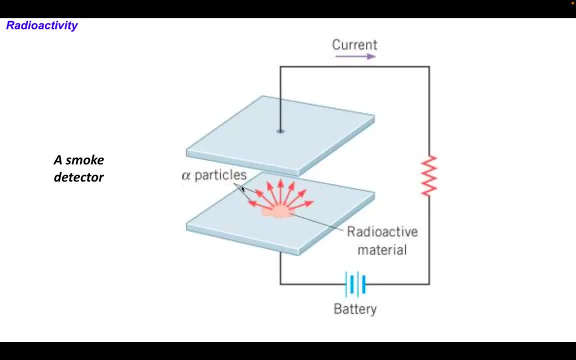 particles is continuously emitted, but if there's a smoke, the alpha particle will be blocked, and if the circuit is blocked it will trigger an alarm saying that I am blocked by a smoke. okay, so don't play with your smoke detector, just leave it there. usually there's maintenance engineers will come to check on it. but 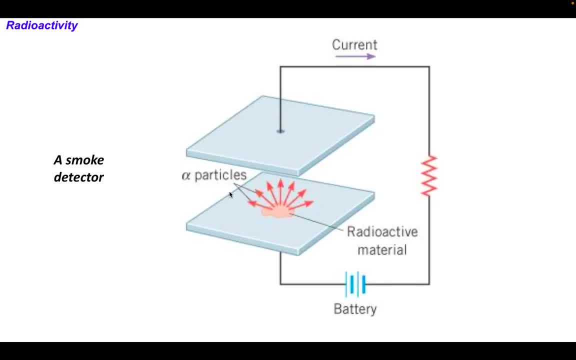 don't play around with your smoke detector. usually alpha particles are, the energy of is deposited in air in a by a few centimeter. so it cannot, you know, hit you, because a few centimeter of air the energy is already deposited in air. okay, unless you take out the radioactive material and put it in your skin so your 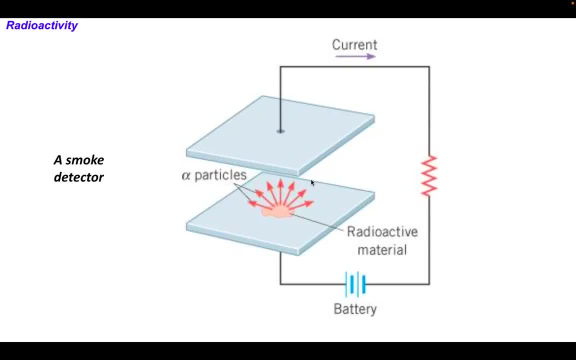 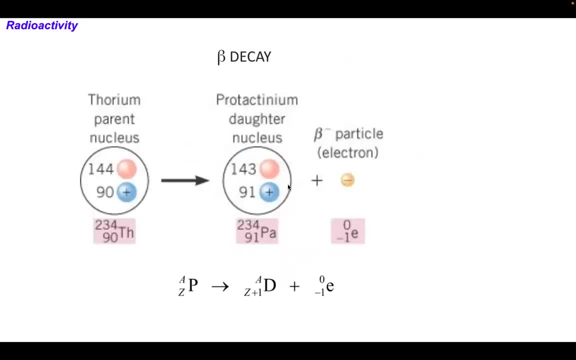 skin might be danger, or your. if you inhale it, the membrane of your lungs will be affected. okay, beta decay. so here you have a parent, let's say for you, it will decay to a daughter and it will emit a beta particle. so here the proton changed, the atomic number is changed plus one, but 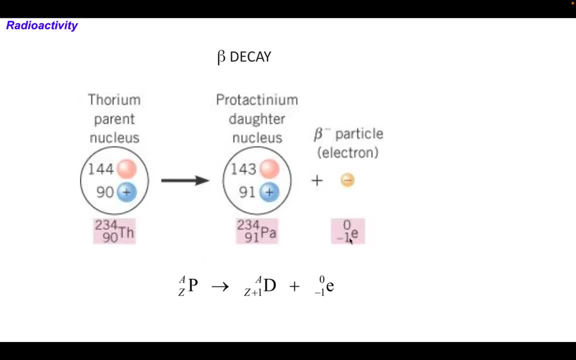 what is happening here is a neutron is converted into a proton and an electron, so added proton and then emitted electron. we're going to check the balancing of the equation there. the same mass number, a atomic number, C, C plus one, minus ones, is there only one: carbon. 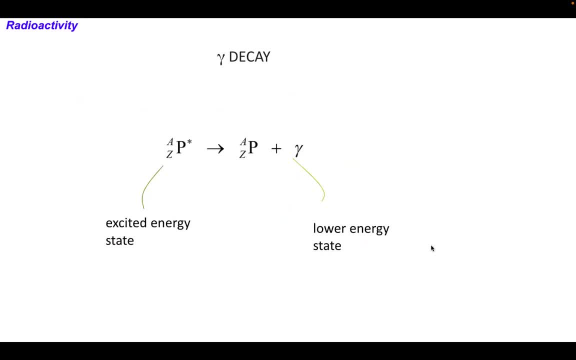 ok, now let's go to a gamma decay gamma radiation. so nothing is changed. elemental: the parent. the daughter is still same element, but with lesser energy, because the excess energy is emitted as a gamma decay, lower state energy now. so this is the excited energy state of your parent. 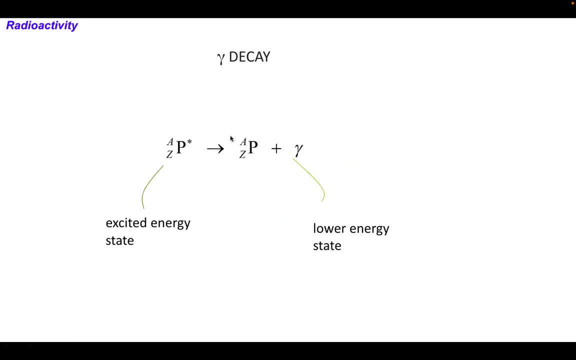 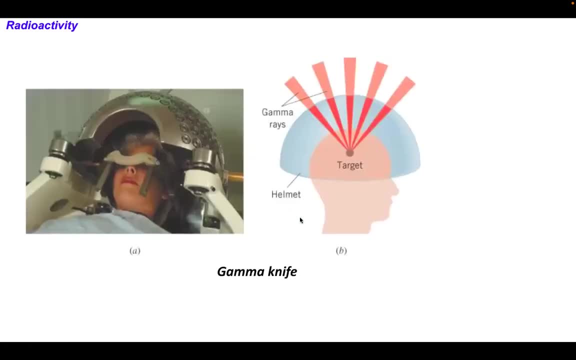 particle radioactive material emits a gamma and then becomes more stable element. okay, so one application of gamma radiation is in cobalt 60 treatment of cancer patient. so this is a brain. we call it the gamma knife because it melts the tumor using gamma radiation like a knife. 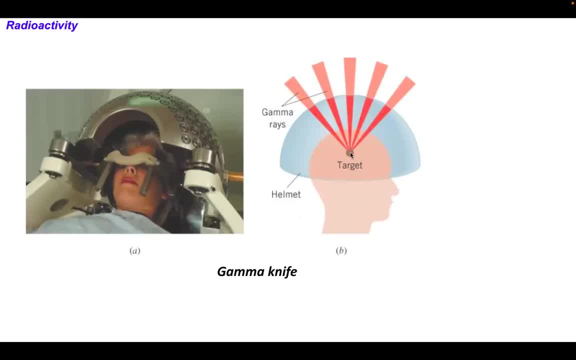 like precisely, you know, hits the target and it will. it will kill the cancer cells and it will melt the tumor, like literally, okay, oops. so take note that this radioactive decay can be a series of decay. so we have a pair of radioactive decay and we have a series of decay. so we have a pair of. 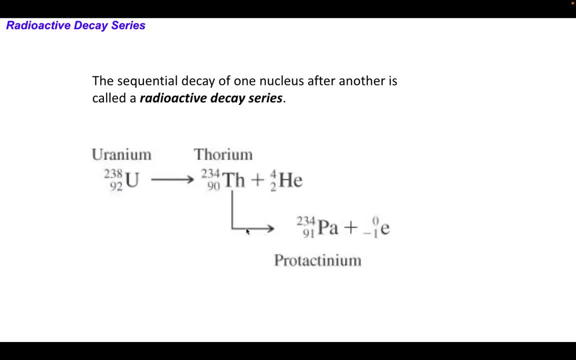 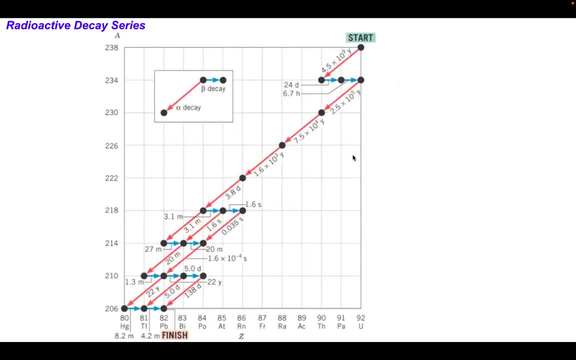 we have a daughter, but thorium is still radioactive, so it still can decay to another daughter- for tactinium in this case- and then it can be a series like this. so, for example, you have uranium alpha decays into thorium and then beta decay into palladium, back to uranium and then uranium. 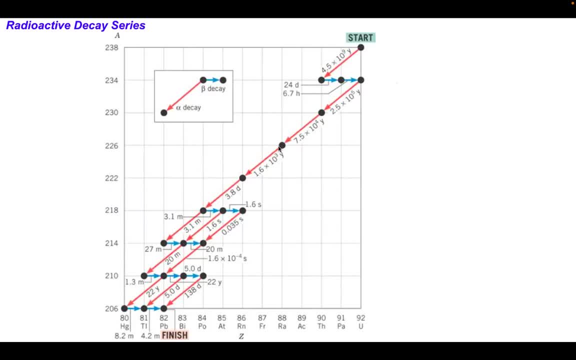 will decay into alpha decay into thorium- check, check, check, check, check, check, check. look at this table: decay into polonium, alpha decay into lead. finished product is lead. but if you go to another series like this, beta decay into beta is blue, beta decay into lead, but it's still radioactive lead, so it still decay. 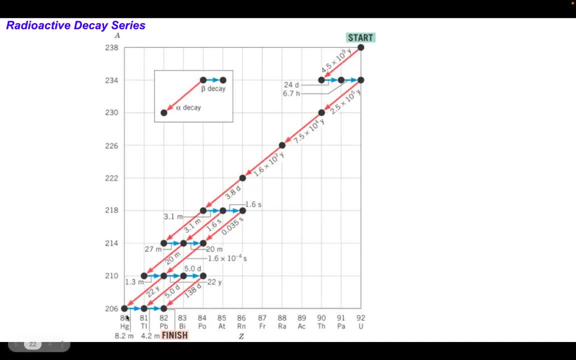 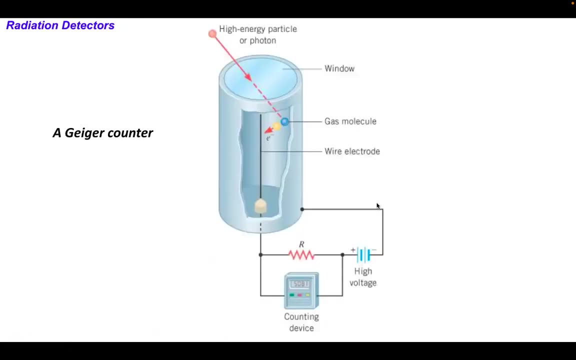 beta or alpha into mercury, uh beta decay into thallium, beta decay into lead, so it can be a series of radioactive decay and every time it decays it emits either gamma beta, beta, gamma beta alpha or even gamma radiation. okay, so how do we detect it? we use a geiger counter. 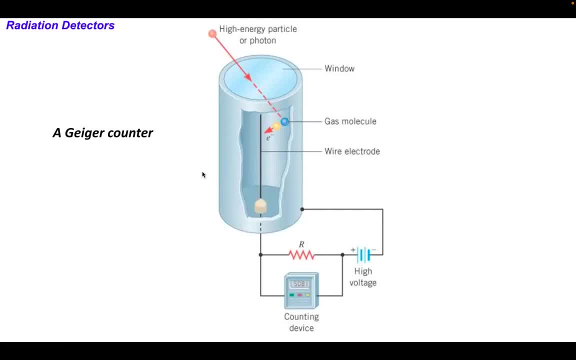 i think if you watch it in some movies there's some sound. sometimes if there are more radiation, it will take it low radiation, so we actually detect it because of its ionization effect. so if you produce, if you produce ions, this is your radiation, ionizing radiation you produce if you. 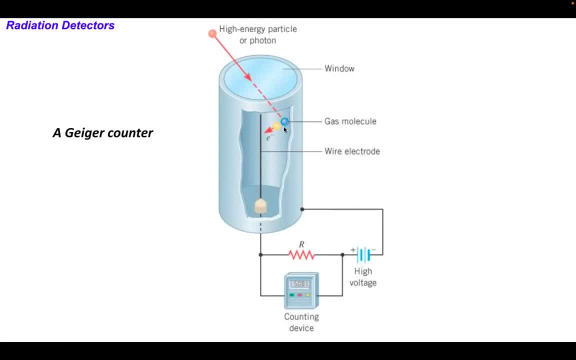 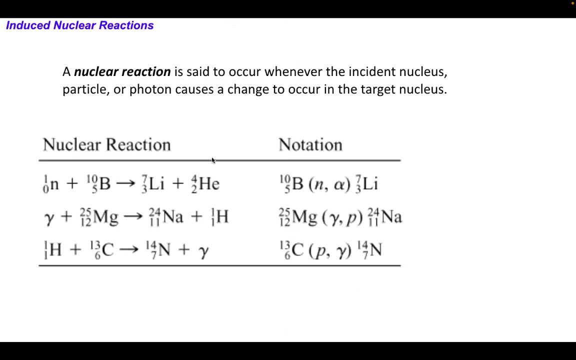 produce is on the sensing part of the device. the electron is collected by a lead and a lead a wire. so on this wire can be uh can, is connected to a counting device or voltmeter, you can measure that, the collected electrons, the current. okay, so that's how. that's how it works. now let's proceed to nuclear reactions. so we're done with radio. 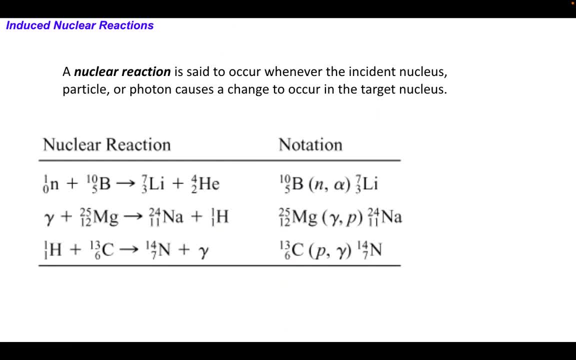 activity. nuclear reaction is you actually bombard a nuclei or an element by a can be a proton, can be a neutron or can be gamma radiation. so like hitting something like a billiard ball: hit something with uh, another something in, in this case, nuclear reaction. you can hit it with a new. 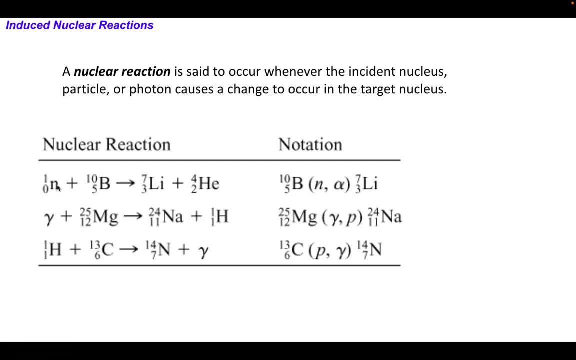 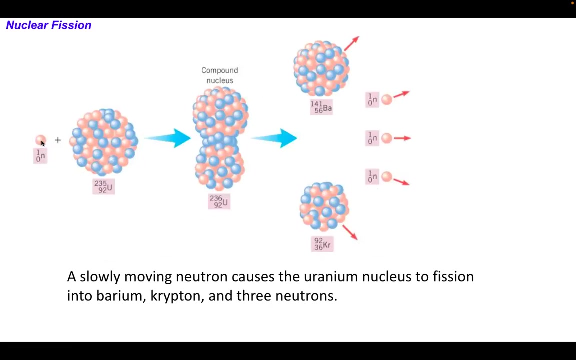 nucleon neutron i mean a gamma or a proton. so if you bombard it with a neutron, the boron will become lithium helium. okay, a nuclear reaction is said to occur whenever the incident nucleus, particle or photon causes a change to occur in the target nucleus. okay, so let's have an example. we have uranium now it is being hit by a neutron. 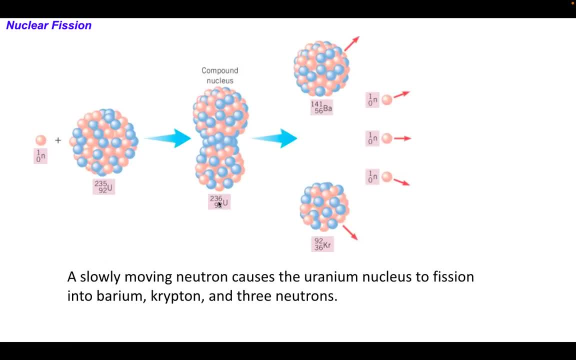 so this uranium will become uranium, two, three, no, no, it will become barium and it will become krypton. so it will split up and in the plus process of splitting up, some of the nucleus are left to uh, left to free, like they are now free. so take note that 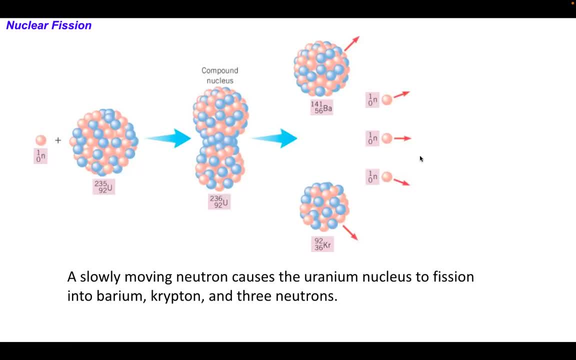 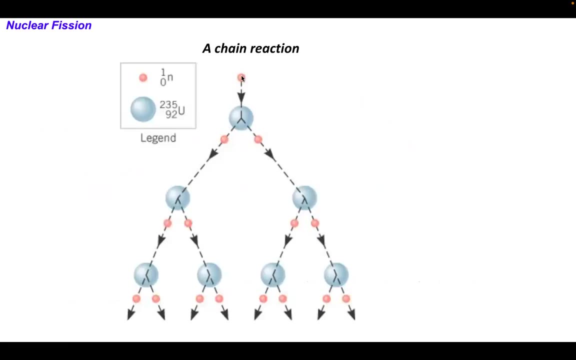 one neutron can actually produce more neutron, so it can be a chain of events. you already produce two more uh elements and, in this example, three more neutrons, so it can be a chain reaction. so one neutron can produce two more more, more more the surrounding uranium can. 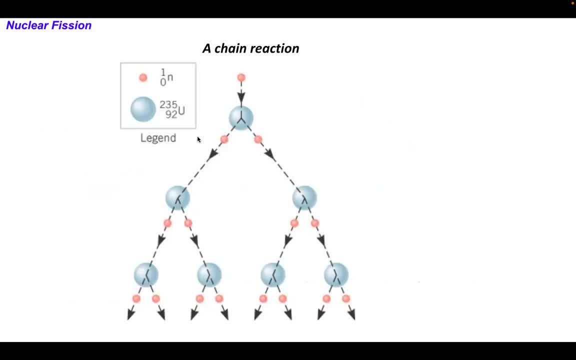 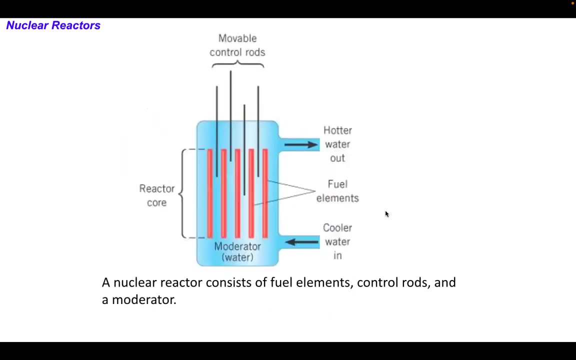 still the. this neutron can still hit the surrounding uranium and then produce the same reaction. it becomes a chain reaction. so it can be an uncontrollable process. but for specific application you have to control that because it will produce tremendous amount of energy and radiation coming out. so in a controlled chain reaction only one neutron or an 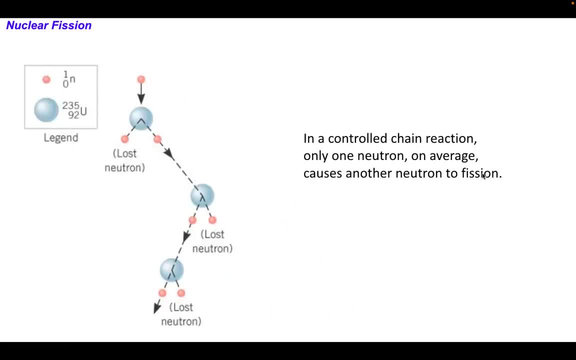 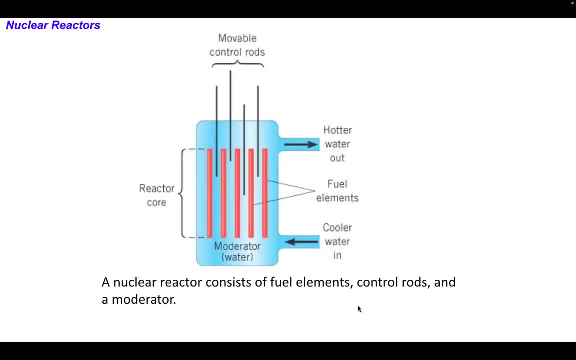 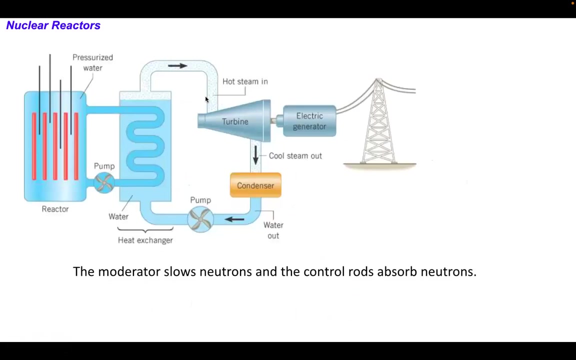 average causes another neutron to fission or split up something. okay, so like in a nuclear reactor. so there are fuel elements, control rods and moderator. so these control rods are the ones that limits the chain reaction of events. okay, so this is your core reactor here. so this is a nuclear reactor in the nuclear power plant. so the reactor core is actually. 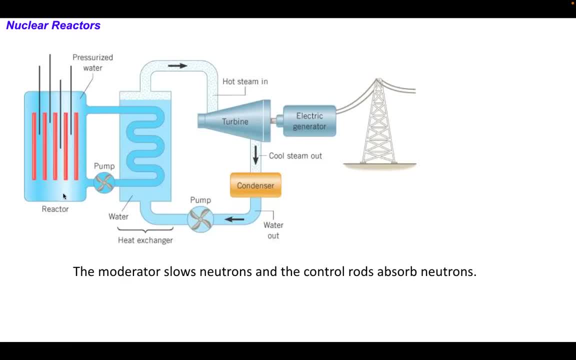 composed of the movable rods to limit the chain reaction. so it's composed of water, another water and water vapor, here condensed. so the moderate moderator slows neutrons and the control rods absorb neutrons. so, oops, now there are concerns of accident, like the ones that happens in. 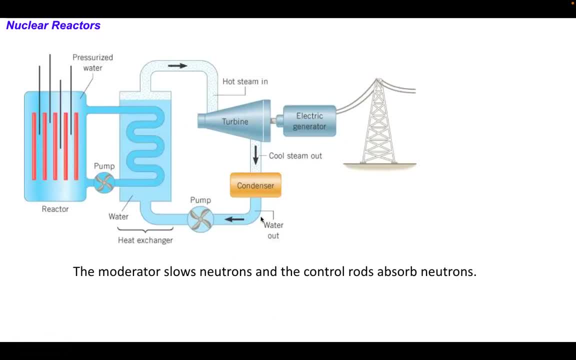 fukushima and daichi, wherein the cooling system was affected by the mead, so it got destroyed and they failed to turn it off or contained it. so if your cooling system is destroyed, then it will just heat up, heat it and it exploded actually, and some of the radioactive 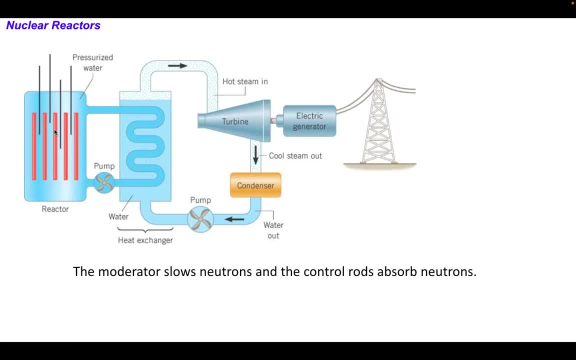 materials escape through the atmosphere to the sewerage. so the whole parts, i think it's like 10 kilometer, and later on one kilometer radius was evacuated, and you know the, the radioactive material. we even detected it in pnri, so it was in the news. so to be so, then the, the modern designs of 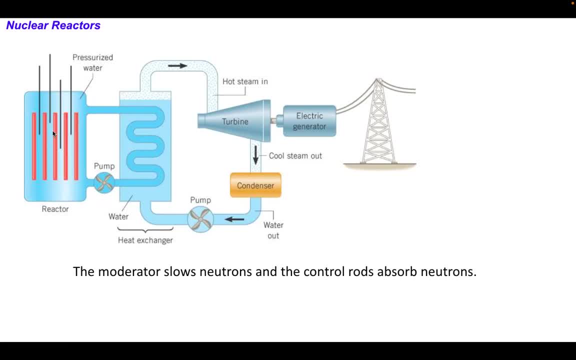 nuclear reactors are actually safer. different design now, smaller modular type. then if there are risk of uh explosion, earthquake, they are failed to safe. they will, you know, under underground so that no radiation or radioactive material can escape through the atmosphere. so it's safer. now the other type of nuclear reaction. so we have nuclear fission, the splitting. 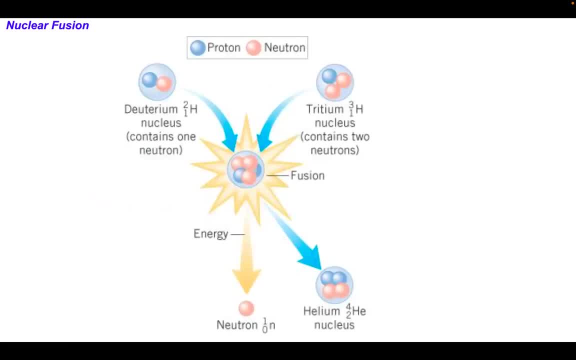 up. the other type is nuclear fusion fusion like in dragon ball z, so vegeta and sangoku. they were fused into one element and in the process of fusion you produce tremendous amount of energy, usually heat. so let's say you have the ethereum and lithium, both hydrogen, then you are going to fuse them and they will fuse and then they will produce. 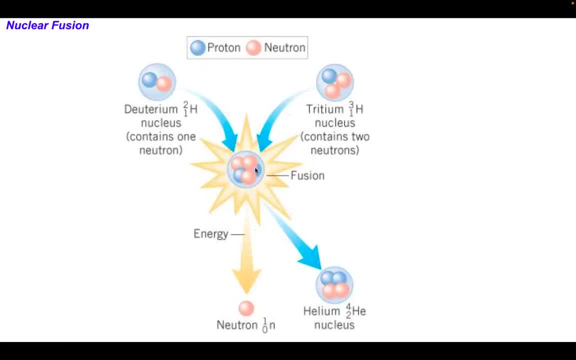 tremendous amount of energy. you will produce helium and heat, heat, heat, lots of heat. this is the process. what is happening in the stars? the sun is like a huge nuclear fusion reactor: tremendous, almost unlimited amount of energy. because of the gravity of the sun, hydrogen are being fused together to produce helium and other. 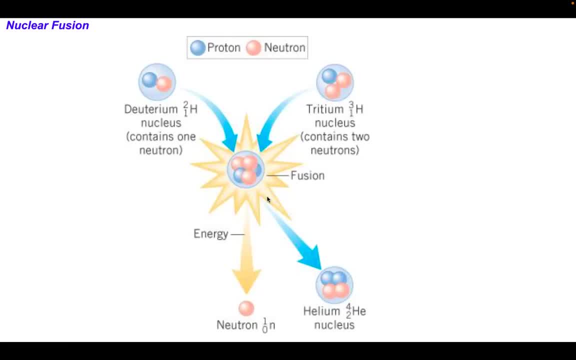 neutron and other forms of energy, mostly heat, and all the range of electromagnetic in electromagnetic spectrum. okay, so it's hard to control this because you need to contain that in the sun. you don't need a containment because we actually are benefiting from the nuclear fusion of the sun. it produces a lot of energy, heat, visible, a lot of energy. 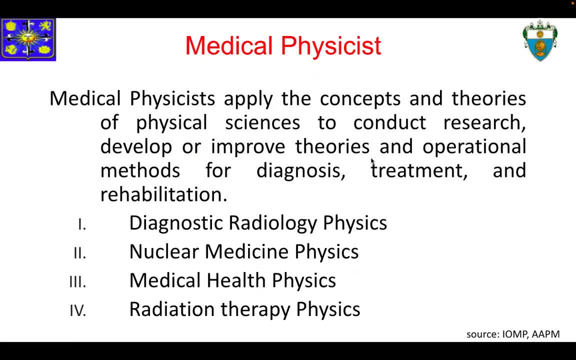 now let's proceed to applications of radiation in medicine. so, as i've said, i'm a medical physicist. so what does a medical physicist do? we apply the concepts and theories of physical sciences to conduct research, develop or improve theories and operational methods for diagnosis, treatment and rehabilitation. so, as a medical physicist, they're actually sub-branches of medical physics. 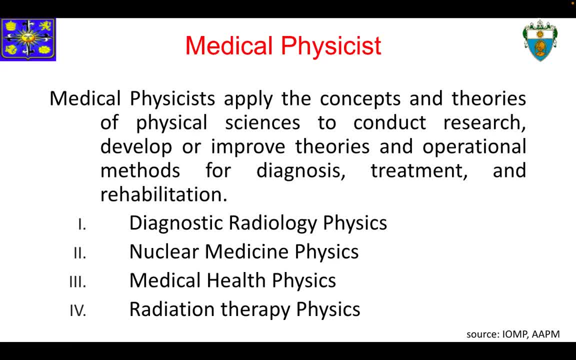 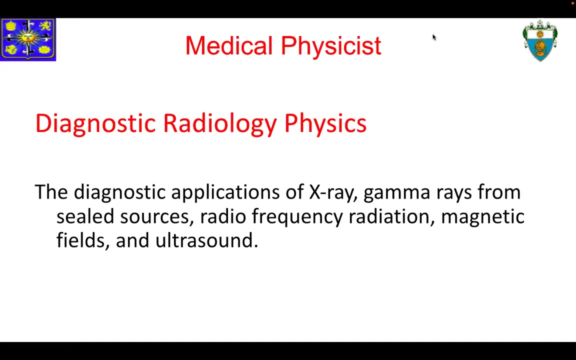 so there are many such principles are included in medicine, вари, stirring, even diagnostic radiology, physics, nuclear medicine, physics, medical health physics and radiation therapy physics. i did some residency for radiation therapy physics but we do have some practicum in diagnostic radiology, nuclear medicine, some medical know okay. so let's go to the first one, diagnostic. 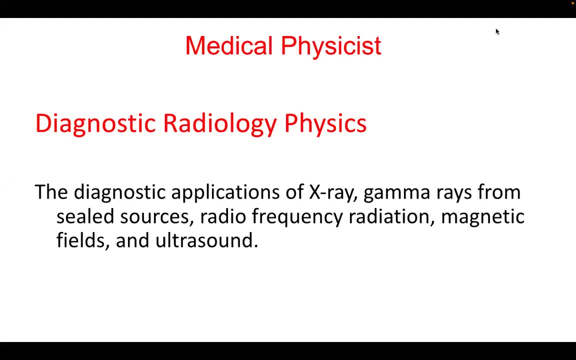 radiology physics. radiology physics: the diagnostic applications of x-rays, gamma rays from sealed sources, sealed radioactive sources, radio frequency radiation, magnetic fields and ultrasound. so the purpose of diagnostic radiology physics is applying physics to diagnose patients, any forms of diseases, to see what's inside the patient. so we use x-ray. so you will encounter machines as an x-ray machine. 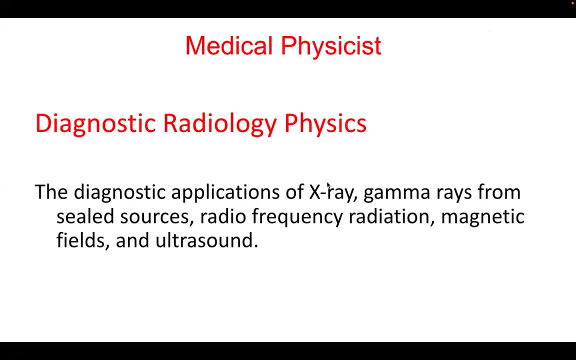 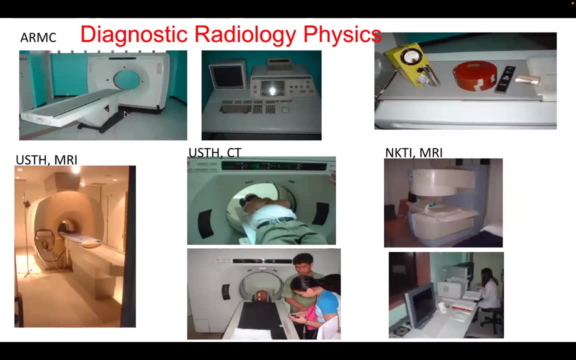 fluoroscopy machine, cp x-ray machines, um. even radio frequency and magnetic mri is part of diagnostic radio radiology physics and ultrasound as well. so here i did some uh practical in among rodriguez medical center. this was. these are my pictures, long, long time ago i think. 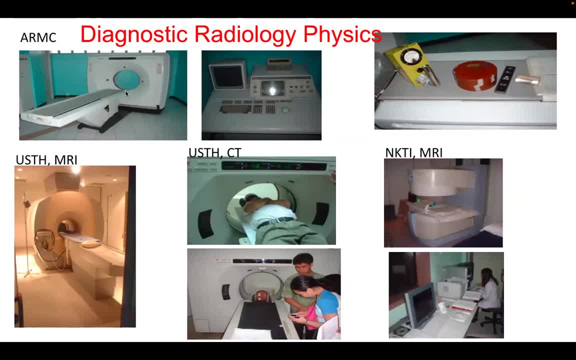 i don't know, 15 years ago or 18 years ago- long time ago- so they might have different machines now, so these are the old ones. so this is the, the ct control console. these are the machines that we use for my undergraduate thesis, so perhaps this is 20 years ago, okay. so this is the geiger counter that we use, and some. 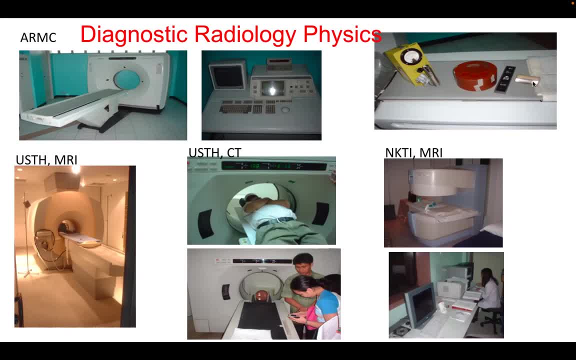 phantom to do some tests and the quality of the image. these are the substitute for the bones, for the spinal cord, for the lungs. so we do some testing and alignment tests and leveling tests. this is the mri- magnetic resonance imaging, which used to image the patient, usually for soft tissue. 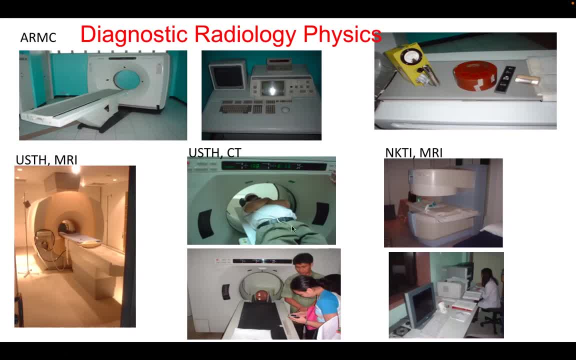 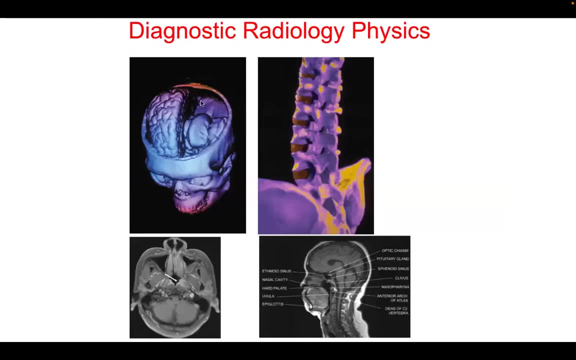 this is in us hospital, mris. it is canned so they have new machines now for ct scan. this is national kidney transplant institute. they're permanent magnet, mri, the control console. so these are sample images of diagnostic radiology. this is ct x-ray cd of the 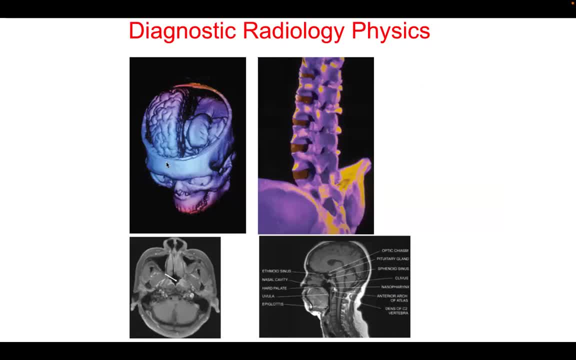 tomography. so, as you can see, that the bone is quite clear and the structure of the brain, see, it's like. i think this: this patient is operated already. half of the brain is, it's gone and uh, spinal cord, as you can see, you can see the bones and the spinal disc. this one is our. 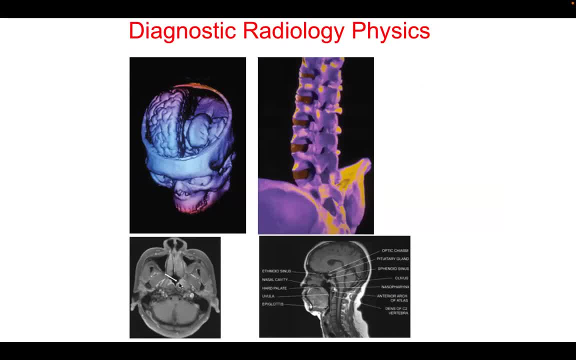 mri images. as you can see, the soft tissues are very clear, but the bone structure are dark. so because of the the physics behind, i'm not going to explain. guys, this is general physics, so we try to want to limit their discussion to simpler, but not simple. if you want to know, or 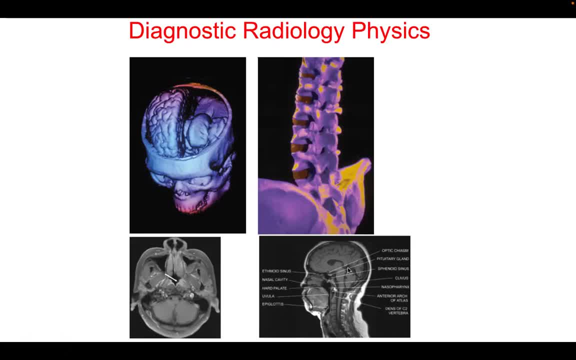 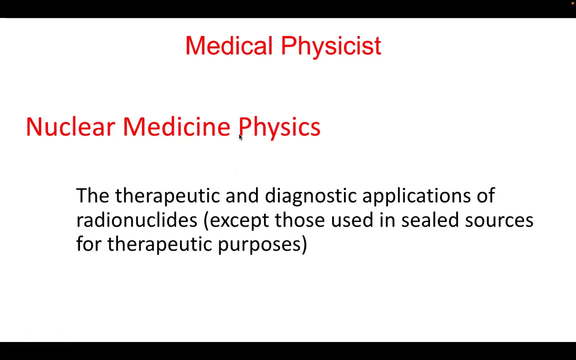 learn more, you can ask me or you can search on your own. so as you can see, the soft tissue, the fatty parts, the hydrogenous parts are clear in mri. next, another branch of medical physics is nuclear medicine. physics a business. you can go to these fields. so in nuclear medicine it's mostly radioactive material. 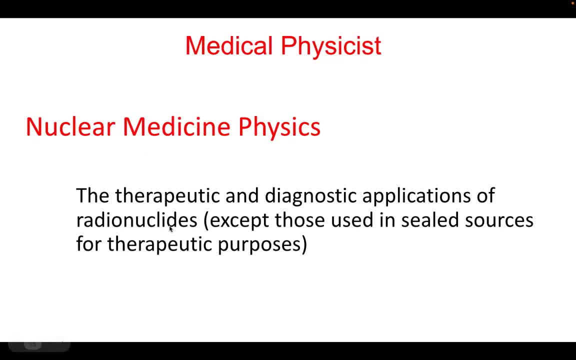 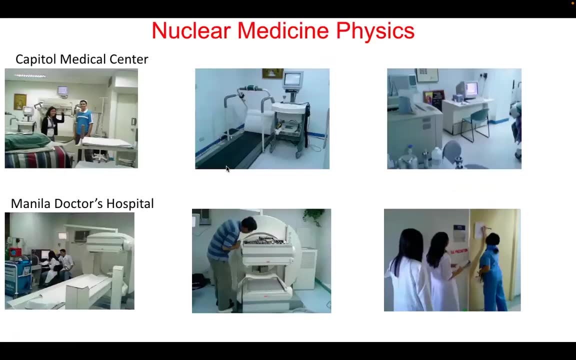 the therapeutic and diagnostic applications of radioactive materials, radionuclides. okay, so both therapy and diagnostic procedure in nuclear medicine. so the the key word here is we use radioactive material, radioactive material. so we did some practical when i did my masters in capital medical center. these are their gamma cameras. 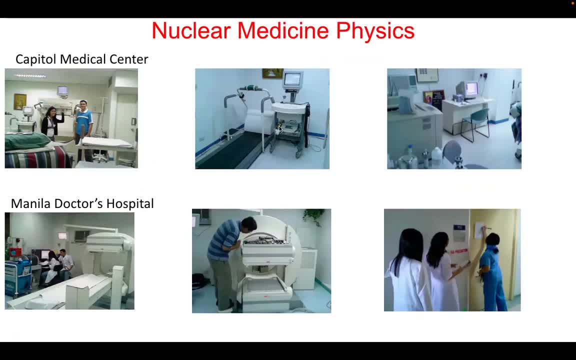 there are some procedures that the patient is asked to exercise for some cardiac procedures and we scan the patient injected or inhaled with radioactive material and that radioactive material usually goes to where the disease part of the body, the tissue, and then we we scan it and here are some engineers who do some repairs or maintenance. 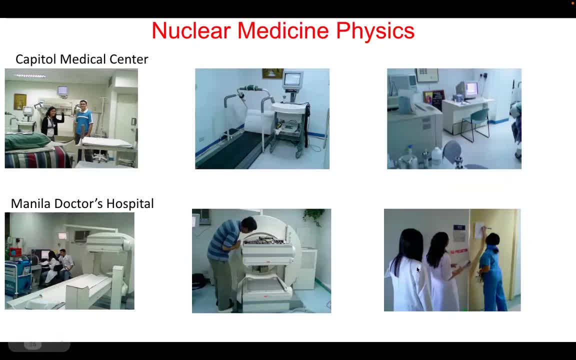 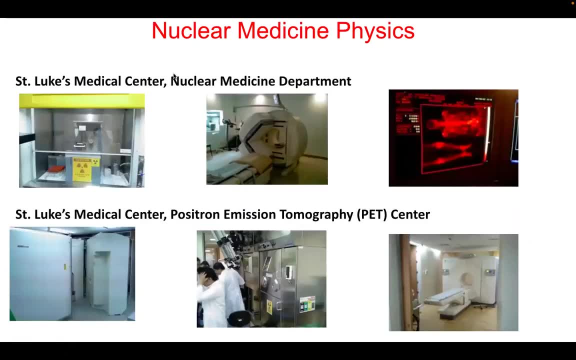 and they're the physicists to measure the radiation outside, surrounding the patient, surrounding the sources. so you have to make sure that we are safe and we use some devices. this is in saint luke's nuclear medicine department. this is where they prepare the radioactive materials. of course it's. 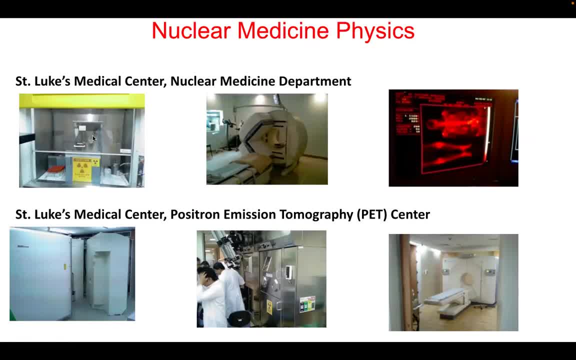 lead shielded, so we are not exposed or the radio pharmacist is not exposed. and this is sample images. as you can see that the cancer spreads to the bone already. we scan it with a gamma camera or the machine and this is for the positron emission tomography. this is in saint luke's. 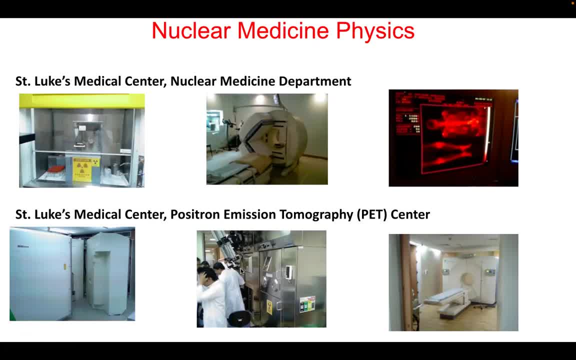 so, as you can see, there's some robotic arm here that is used to to handle radioactive materials. we are not exposed, and this is the pet scan, the positron emission tomography machine, and here i am holding for picture taking. i'm not actually operating it, but 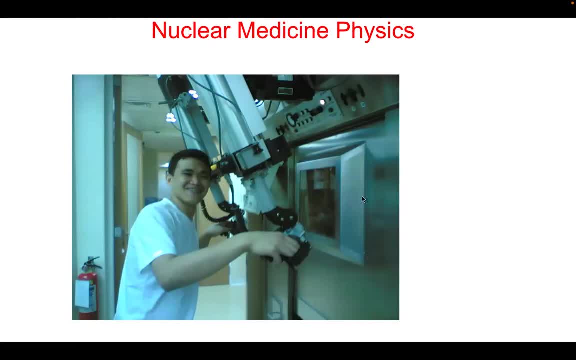 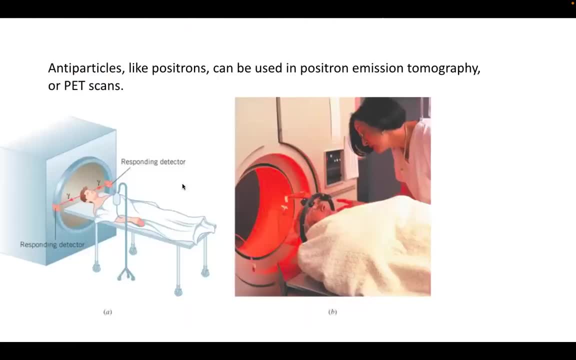 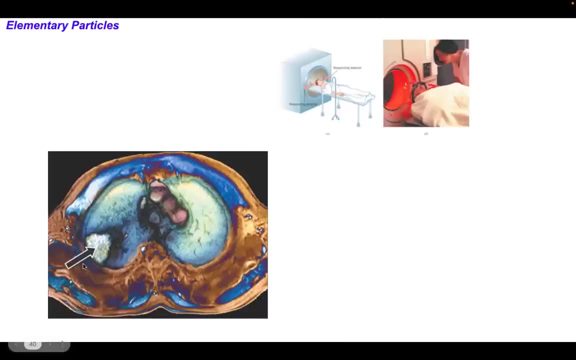 you can see there are some like uh inside the radioactive material, of course, and there is like another robotic arm that handles the radioactive material. so this is her pet scanner and sample images of the pet scan. so, oops, so take note that in most procedures for nuclear 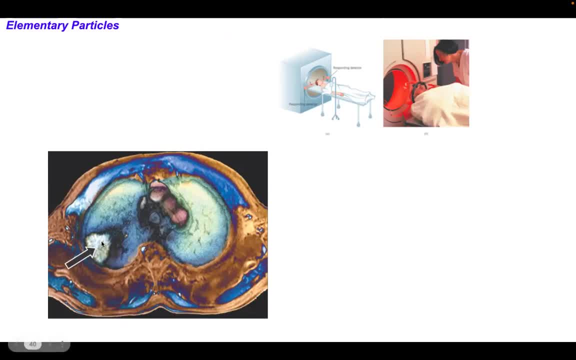 medicine. we can see the function of the functional. we can get functional information of the tumor, of the diseased part of the patient. so this seems to take up a lot of the time, a lot of uh for for pet. it takes up a lot of radioactive material, the flora dioxide and 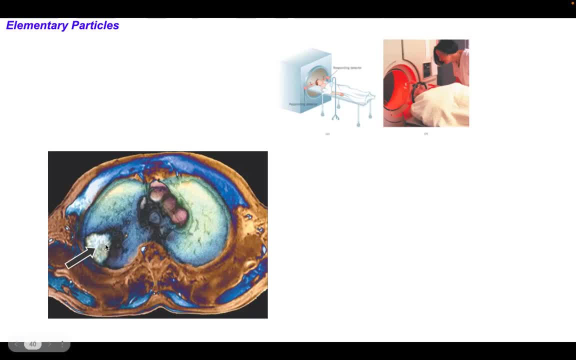 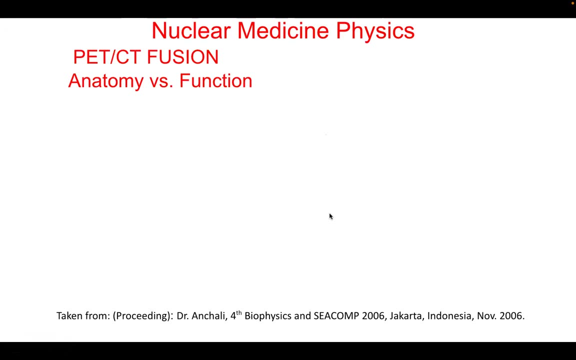 fdg. okay, just search on your own if you want to know more, because we don't have time. this is general physics series. so the radioactive material goes to the tumor part of the lung. it's highly active, but nowadays the trend is you can actually fuse ct, which is anatomical image, and pet, which is mostly functional. so you have. 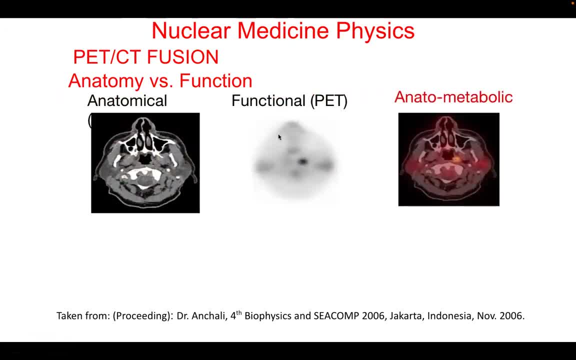 ct scan, here fused with pet, it's a little bit large. spectrally you cannot see much of the structure, but if you combine the functional and anatomical and not the metabolic image, you can see that there are. you can see clearly which part of the tumor is highly active and there are some. 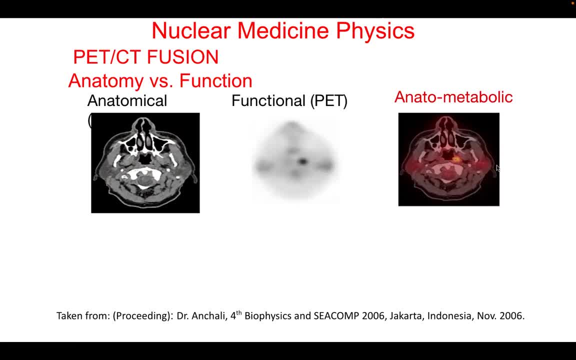 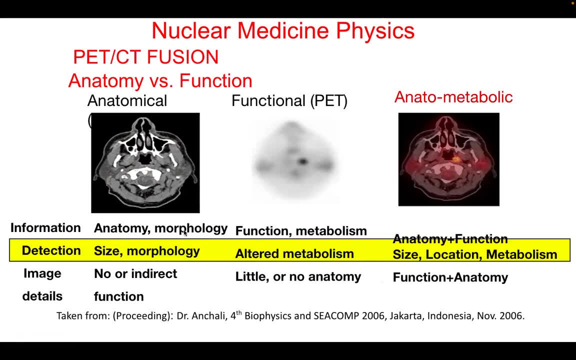 parts who are active here, the sides, so perhaps the lymph nodes are active. okay, so you can get a lot of information for anatomy, the size, morphology, but no function. but for pet you can get the metabolism. so if you combine the images you can get the functional and anatomical image information of the patient. another example here: 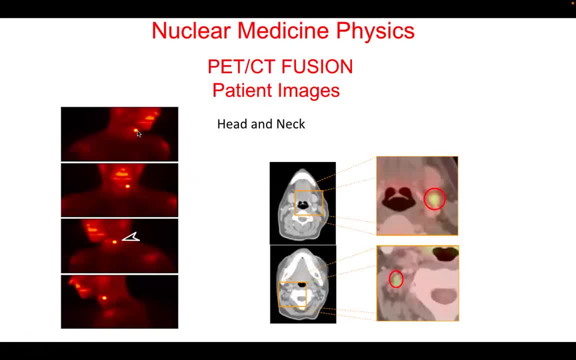 pet ct fusion. these are pet image. you can see where the the tumor is, but it's not that clear where, specifically because of unclear uh structure. but if you combine it with ct you can now see that oh, this is where it is. so that's what's better. oops, you have the ct scan combined with pet images. 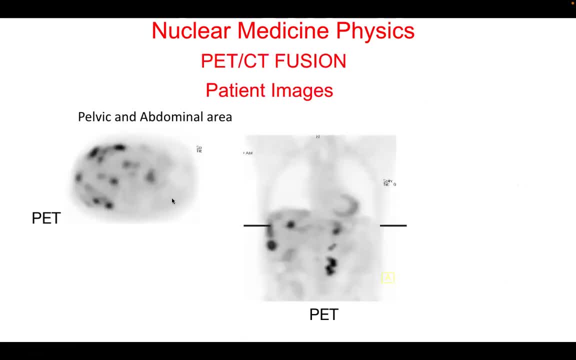 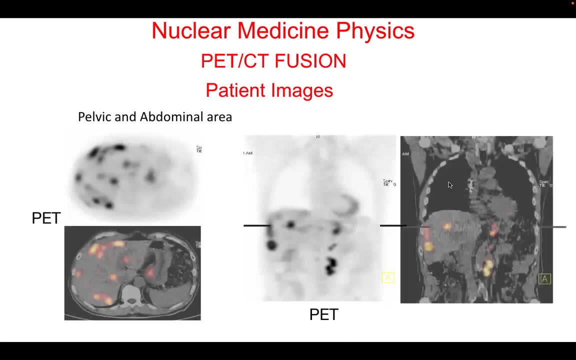 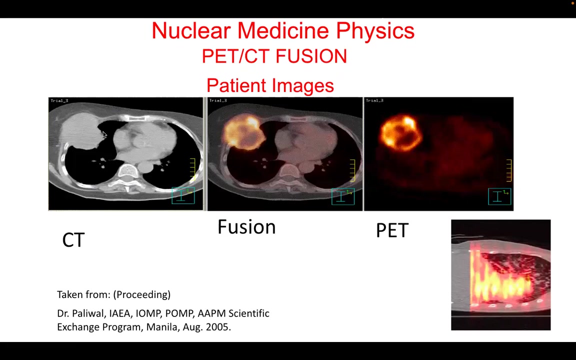 okay, the pelvic area pet images. you can see the function, the uh, it's metastasis. it's metastasis already in the liver domino part, but combined with ct is even better. you can diagnose more accurately where the tumors are. ct: as you can see, there's no information as to the activity of this tumor, but it's in. 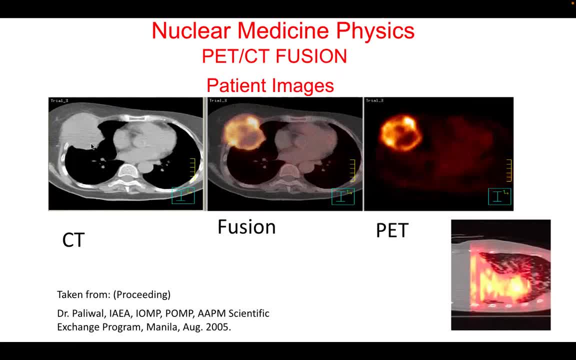 it's already heating up some part of the the lungs. it's a little bit scary already but, as you can see, not all parts of the tumor are uniformly active. some parts of it are highly dividing or highly active. so perhaps if you treat it with radiation you melt it with radiation. perhaps you can give. 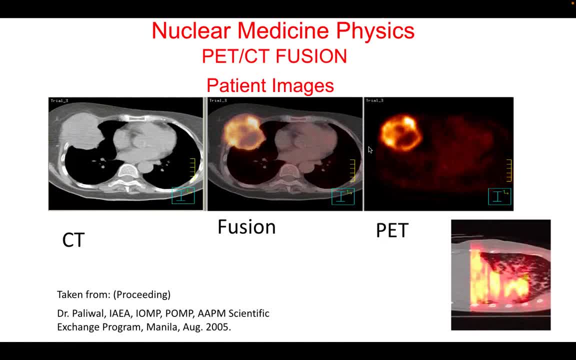 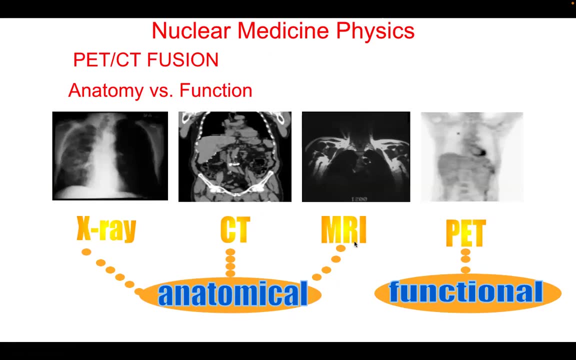 more intensity or amount here, okay. so nowadays you're going to have more patients who are more you can. it's 4d, even 4d, four dimension. this is when you're breathing. you can see the motion. so anatomy plus fusion, these are not high-tech genes. x-ray, ct, mri are more anatomical but pet. 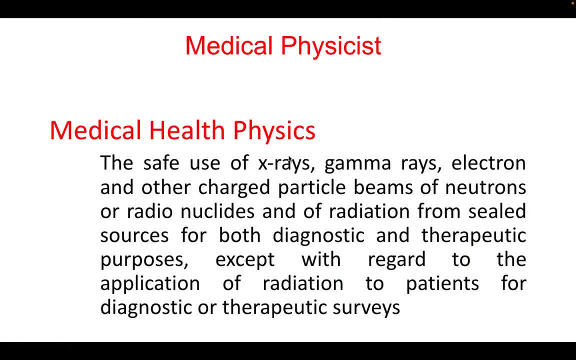 is more functional. now what are the other works or fields of medical physics in the hospital? there's also called health physics or medical health physics, so it's more on the safe use of x-rays, gamma rays, electron and other charged particle beams of neutrons for radionuclides. 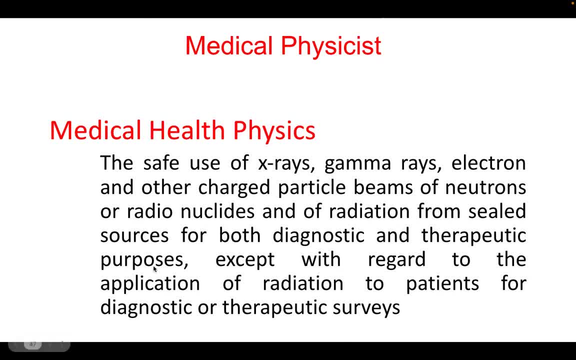 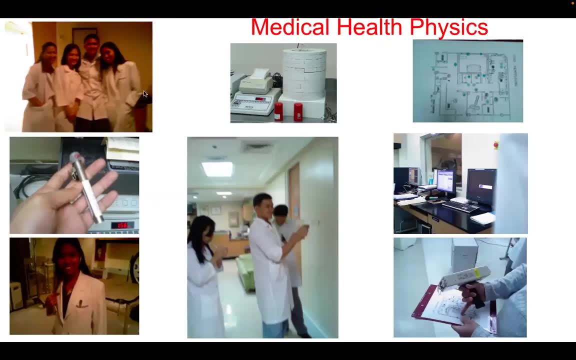 and radiation from sealed sources for both diagnostic and therapeutic purposes, except with regard to the application of radiation to patients for diagnostic improvement. so usually this is more for the safety of the patient and the staff as well. so we are in medical health physics, we're monitoring the radiation dose received by the, the medical physics, but 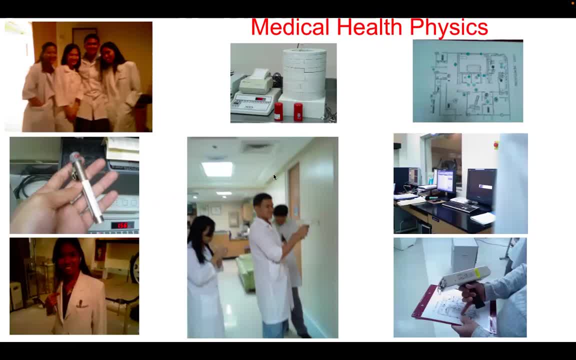 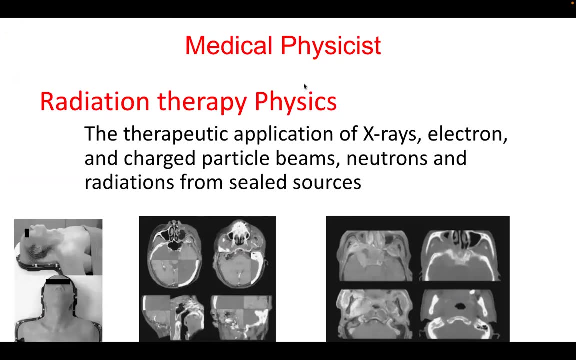 the staff, all the staff, rads x, doctors who are working in these facilities. so we have to check we're receiving too much radiation. they should not. okay, we should not put a risk for unnecessary exposure. and the last part that i'm going to discuss about the fields of medical physics, applying physics and medicine. 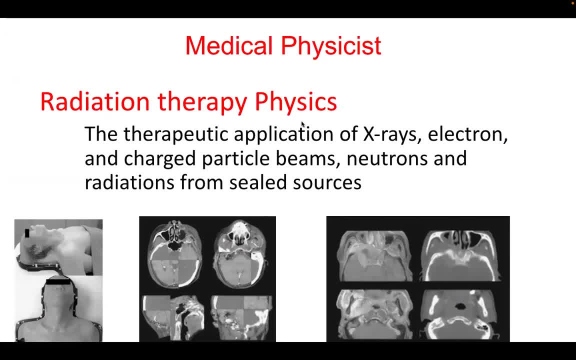 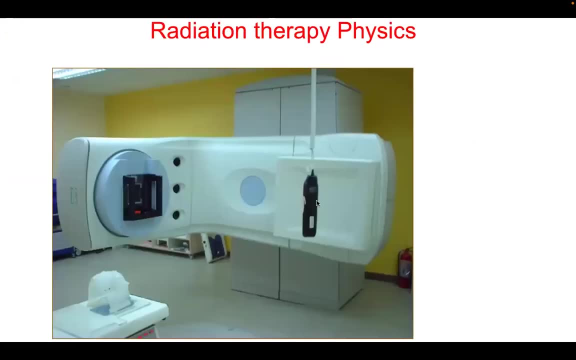 is radiation oncology physics or the radiation therapy physics, so it's the therapeutic application of x-rays, electrons and charged particle beams, neutrons and radiations from sealed sources, usually to treat tumors, to treat cancer patients, so like gamma knife. so this is a linear accelerator. it 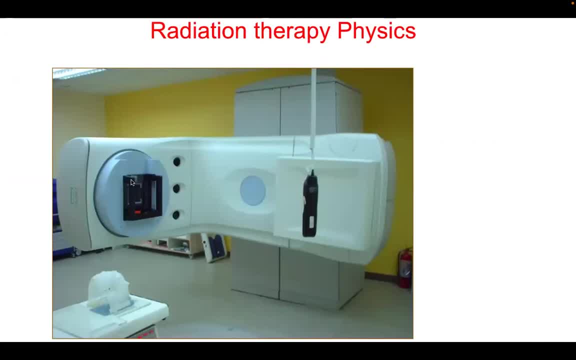 produces higher energy, highly energetic x-rays, so this one is radioactive material. this one is x-ray machine, so we use radioactive material. it emits gamma radiation to treat cancer patients with a tumor, but you can also use much, much higher energy x-rays to treat cancer patients. so we have here: 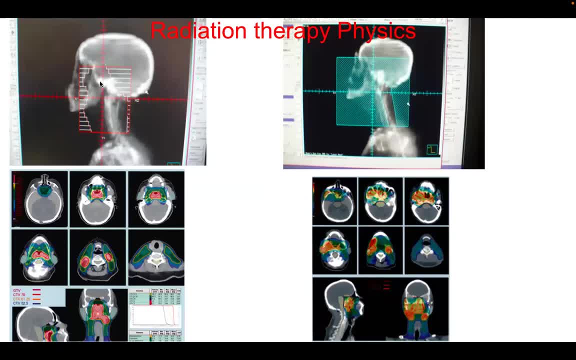 a cancer that is in the nasopharynx, nasopharyngeal area, so that the red parts are receiving hundred percent of the radiation but the blue part is usually lower dose, twenty percent, ten percent, even five percent only. so we're sparing the normal structures of delivering the maximum dose or the 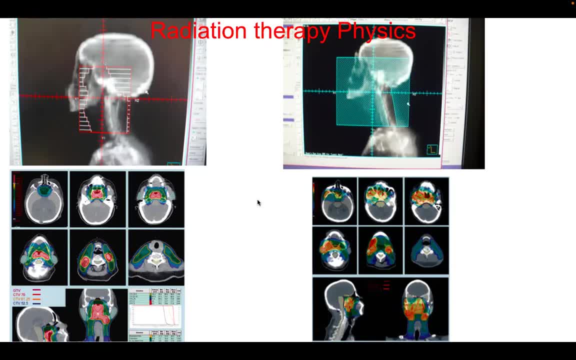 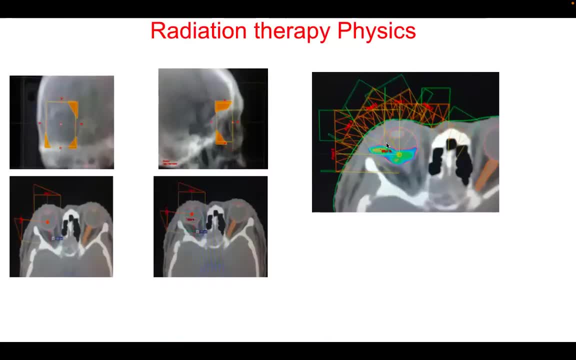 prescribed dose to the target, to the tumor and it's ct. you know, 3d imaging guided. so here, if you have a case, this is retinoblastoma, that like there's like a cancer of the retina. so it's very critical because you you know, there's a high risk that the patient will be blinded. but 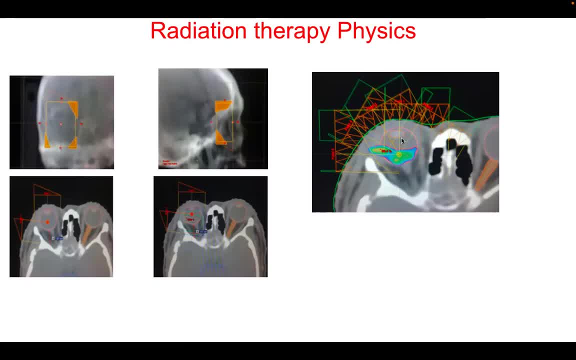 you cannot just let it, you know, grow. definitely the patient will will die because of that. so we have to treat that, that cancer, but as much as possible we have to spare the other lens, the other eyes, and even spare the lens here, because perhaps if the retina can recover and perhaps there's a chance that the patient can still see. on this, 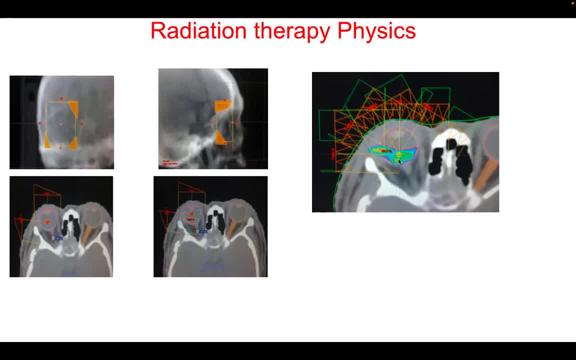 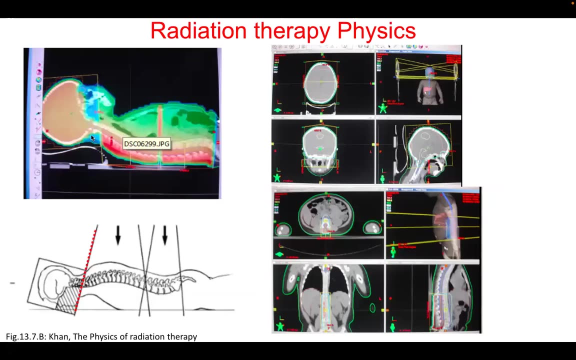 part of the eye. so we have to treat the cancer, the tumor and still, you know, try our best as a medical thesis to spare the lens and other normal structures. it's a very critical case. here. you have a child under undergoing a whole brain irradiation and spinal cord irradiation. so it means